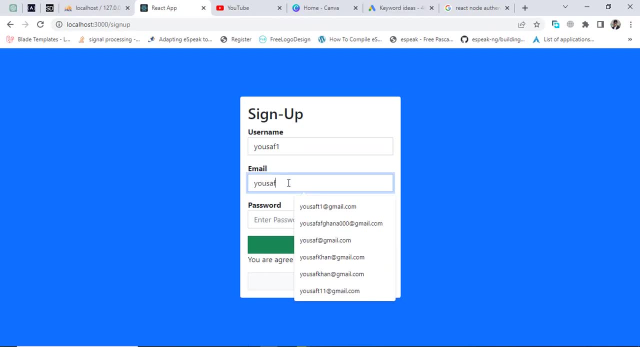 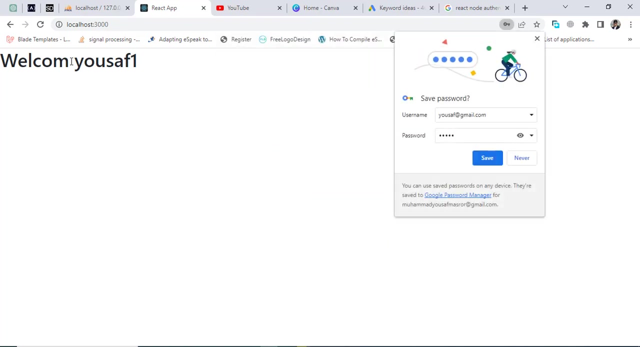 Usuf1 and email usuf at gmailcom and password 12345.. Okay, let's sign up. See, we sign up Automatically. we came to login page, So let's login now At gmailcom, 12345.. Let's login. See, we came and we logged in Usuf1, our username showed to us. okay, So it is our username which is showed. But if we 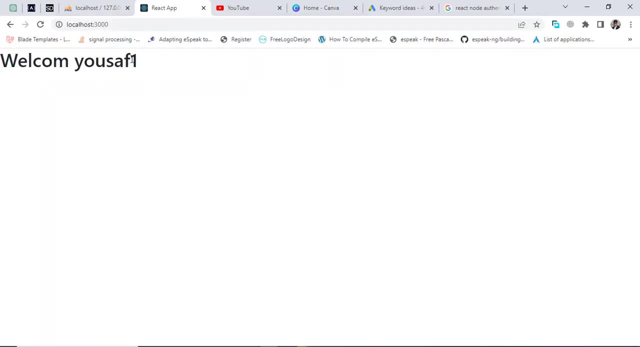 would like now to access our login page. we will directly come to our homepage because we are already logged in, The session and the cookies are set already, okay, So we will perform these functionalities with session and the cookies. okay, So let's get started. 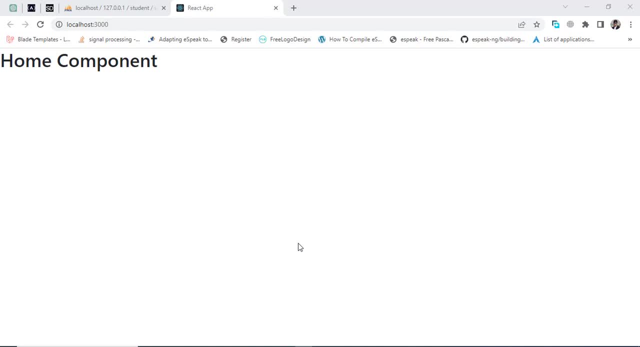 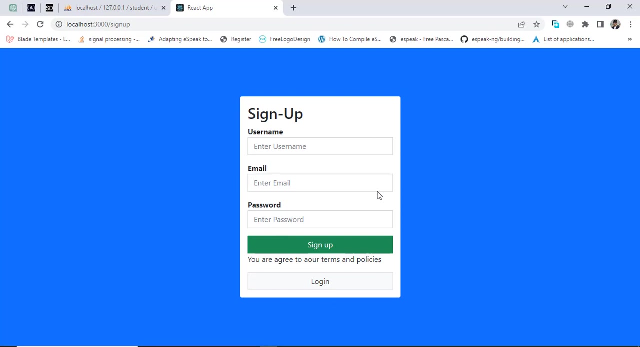 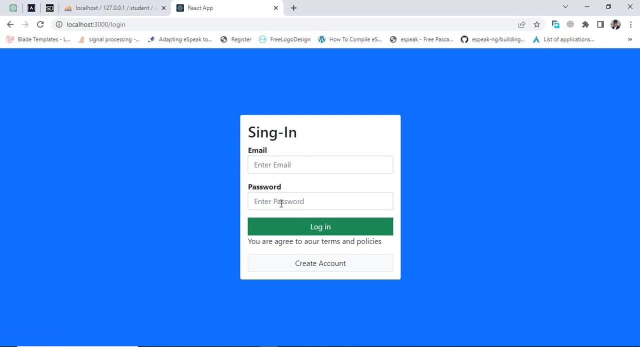 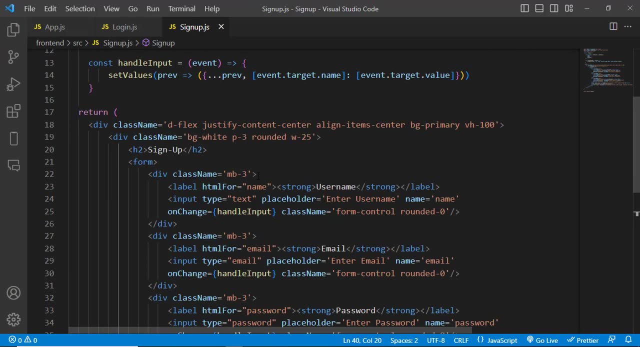 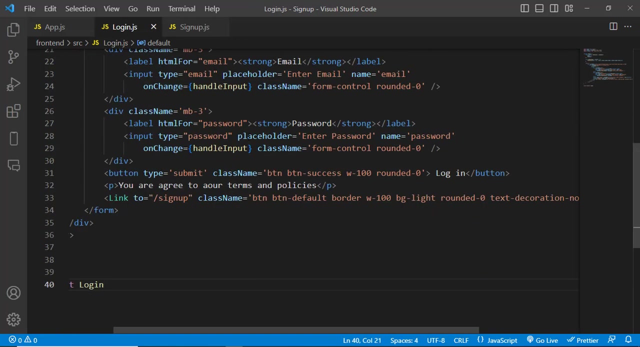 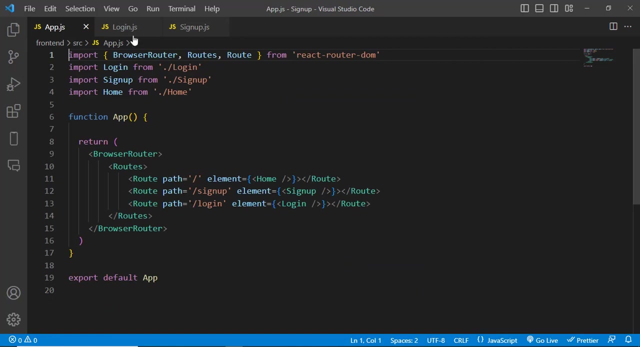 register this account and how to again login and check that. is that exist or not? okay, Let's check first of all the code of this. This is the signup page code. okay, Just simple. okay, This is the signup page which I have written. I use bootstrap for the designing- okay, Very simple. And this is the login which I have used- okay, And also, I have used react router for routing- okay, For slash home signup is login, okay. So now, first of all, let's come to the signup page. 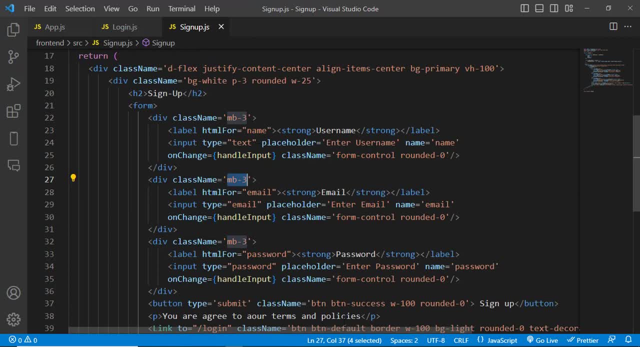 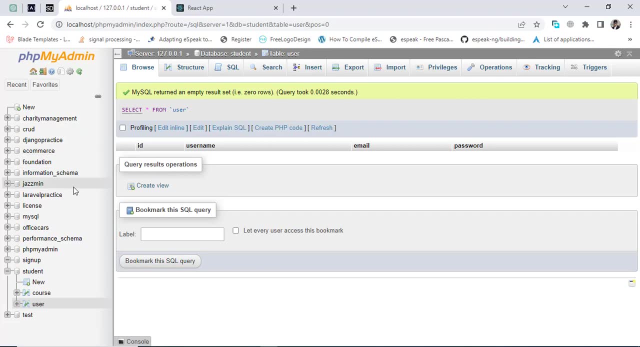 We should register our account in the database MySQL database For the MySQL. I am using this. okay, phpMyAdmin, some server. I would like to store my users here in the signup. I have a table, a database, named signup. okay, Let's check that. 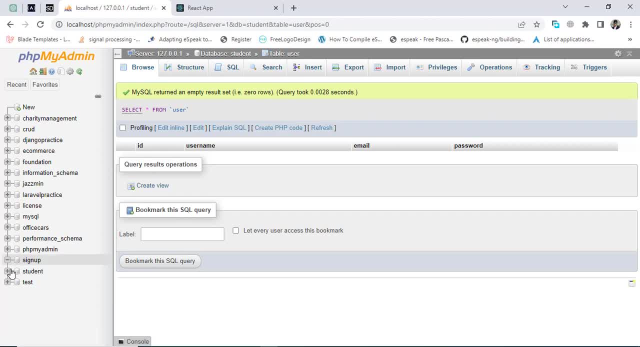 So this come to the signup. We don't have. oh, I think I created that in the. yeah, the student. We will come to the student database and to the user. actually, I will create this in the user to the in the signup. 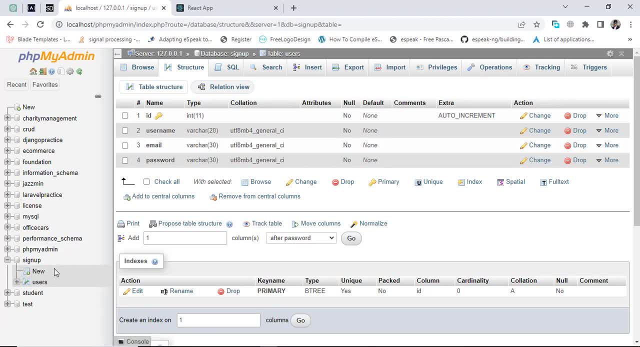 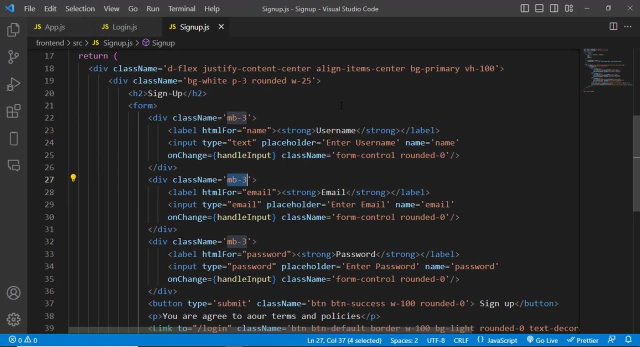 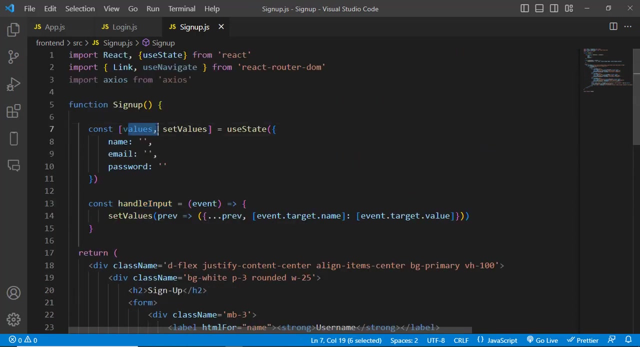 Yeah, I have created the users table inside the signup database, So now let's move to our signup page and to register a user in this table. okay, users, So let's get started. So, first of all, whenever we enter something or some value in this input field in the user name, so that should be stored in a variable. okay, We have created this values object here and we have three pairs in that name: email and password. 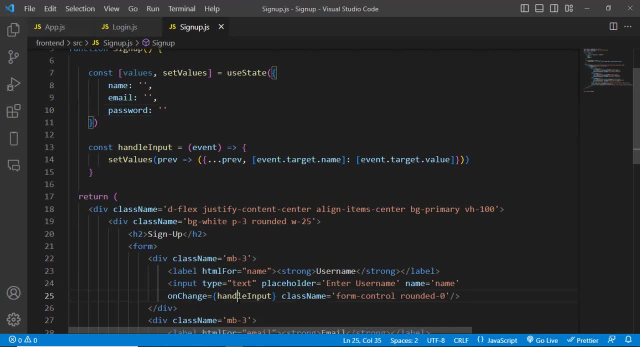 Whenever we enter the values here. so it will call handleInput method: okay, handleInput method, And it will store. update this values object: okay, It will. for update that object. it will call this function And then update the values. 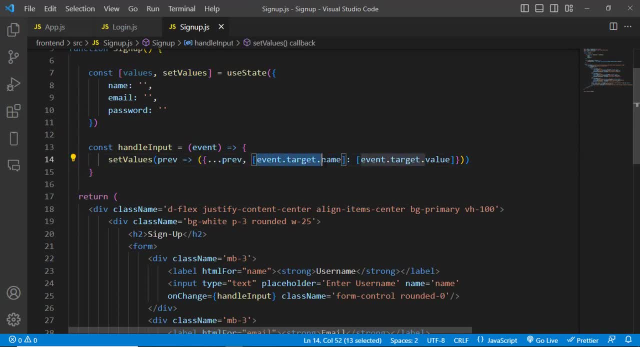 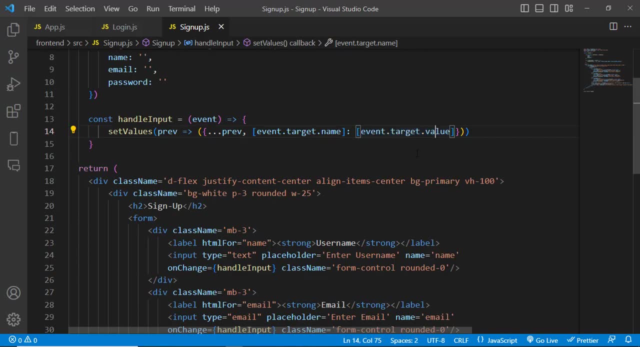 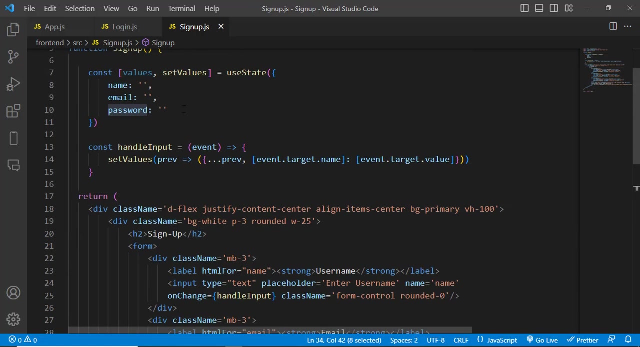 that the previous video with us, then it will update even the target, that name, for example. the name is named with us, so it will update this name. okay, in the same day, winter target data video that we are writing in this input field, same for the this email in the password after our storing our videos inside this. so 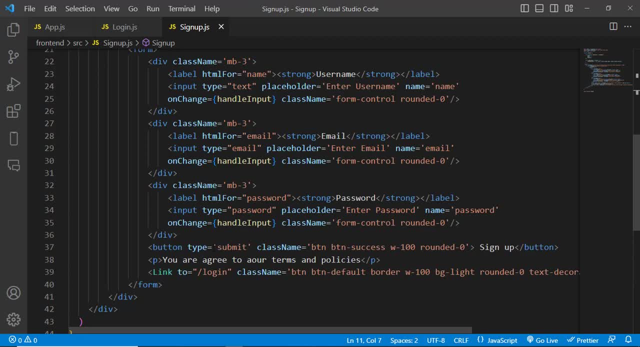 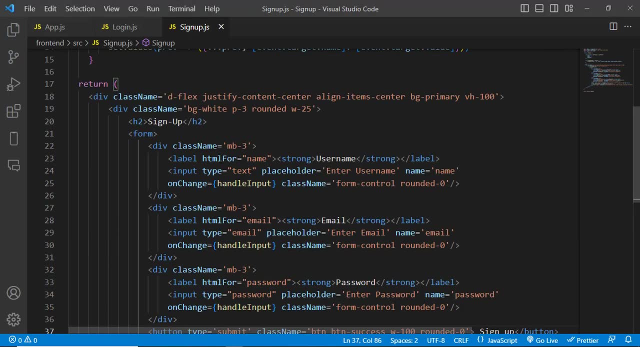 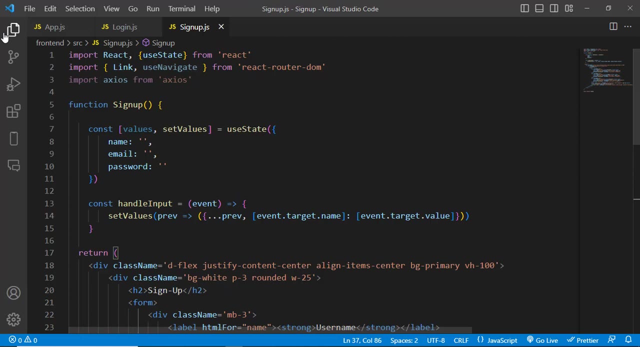 now, whenever we please, this submit will submit button. okay. this submit button. okay, sign up in. your request is submitted. we should pass our data to the server side or to the nodejs to store that in the my, my sequel. so first we will create the environment for our server side at the back end. okay, for the. 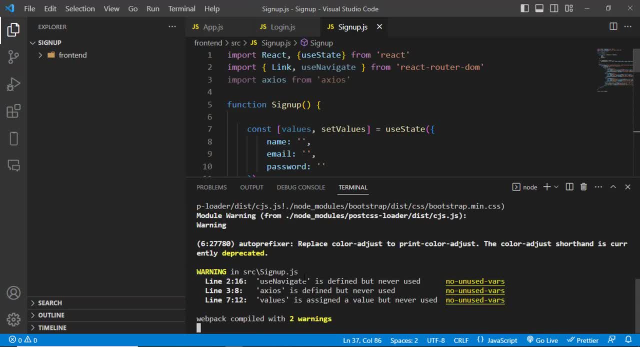 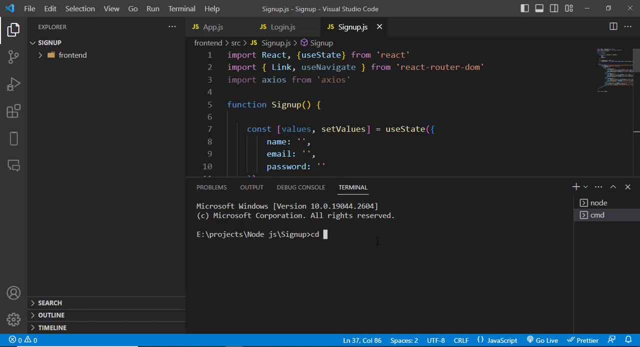 nodejs for that environment. so let's come to the console. let's create a new one. inside this. I will create first of all a new folder, cd server. sorry, yeah, a new folder has created, so inside that I will write npm. let's move to the cd server and npm init. it will create a new packagejson file inside this. 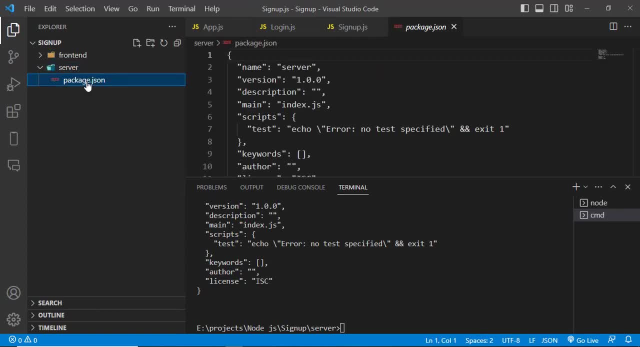 see, let's check it. yeah, that has created. so now let's install a few packages. so first of all we should install npm, install my sequel, express. express is nodejs framework which we will use to for inside, for the backend language. okay, and in my sequel, my sequel is our database. after that course, the cars are. 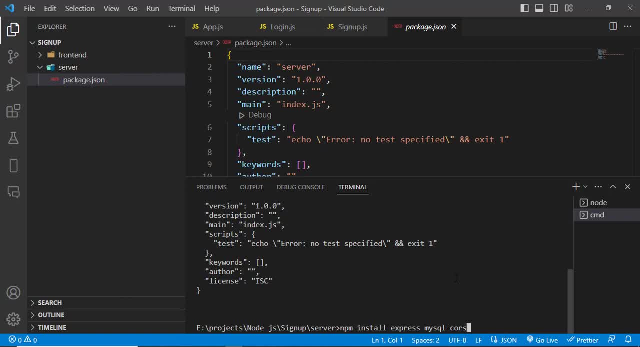 cross origin. okay, for example, we are accessing our server side code inside our fronting, so we should use the course for that, and that's not one, not one is used to refresh our server side code automatically whenever we make some changes inside that, so let's enter, we will install these first. 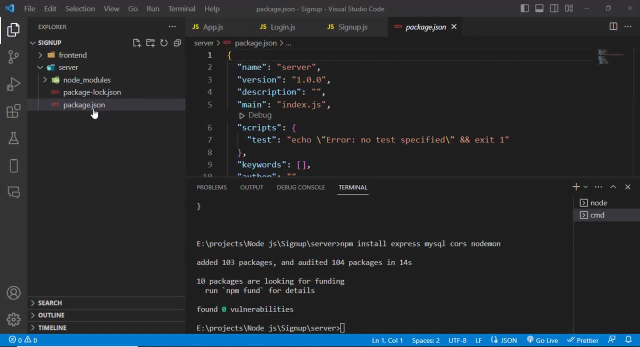 yeah, this is installing. yeah, the packages are installed inside that. so now let's create a new folder inside this, a new file. sorry, the file would be like dbjs. okay, we will use this to write our code inside this. okay, we will write our nodejs with our express. 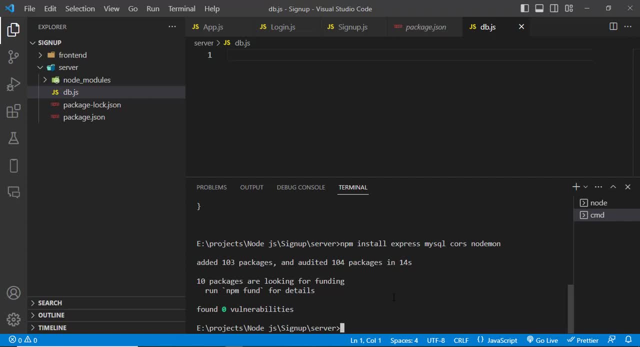 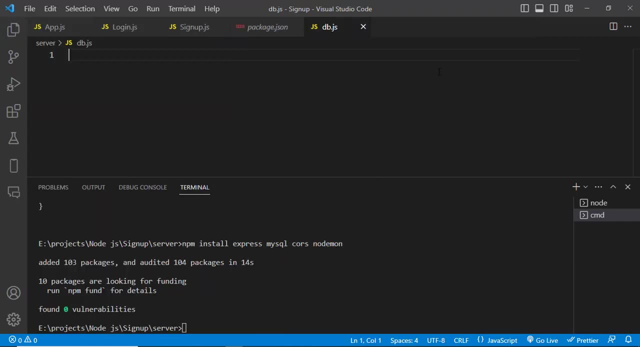 code inside this dbjs. so the initial things that we should write in this dbjs file, those are: first, we should import the Express. to import the Express, we can write now, right like this: okay, const express is equal to require express, but isn't? it is a traditional way. 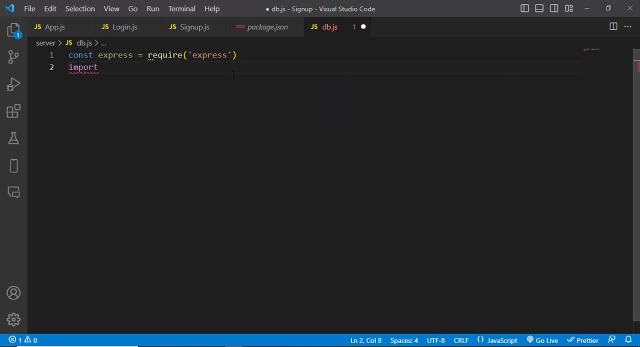 so to write like this: okay, import express from express. so let's check it first of all. is that work or not? up that lesson? sorry, we should write: const up is equal to express. here we should assign a port number. our server will listen on port number 8081. so let's create a function and inside that we 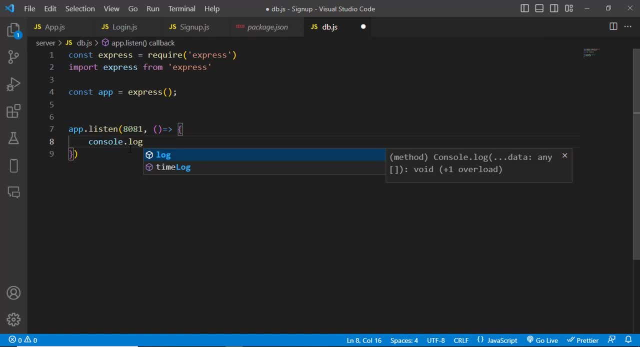 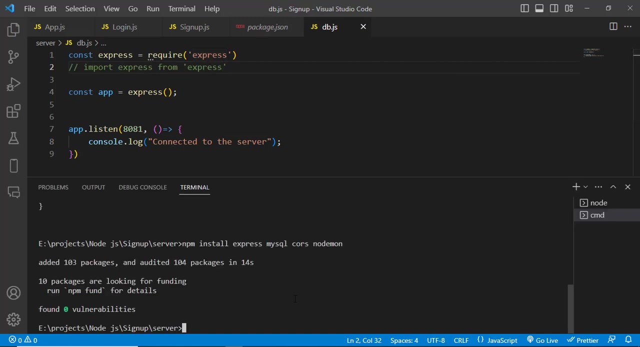 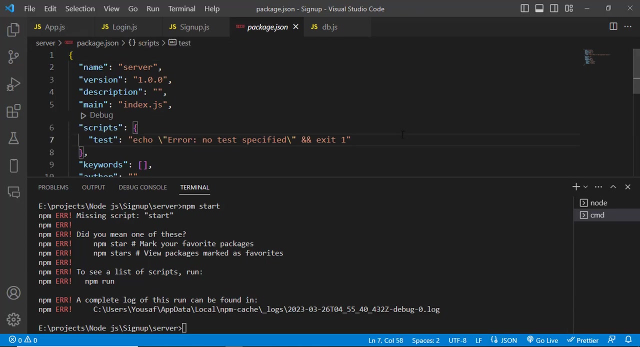 will console dot log to the server. I will commit this one and I will learn our application. let's come here and npm start. we should set up our nerdmon. so for the nerdmon, I will come here and I will write start nerdmon dbjs. let's write npm start. 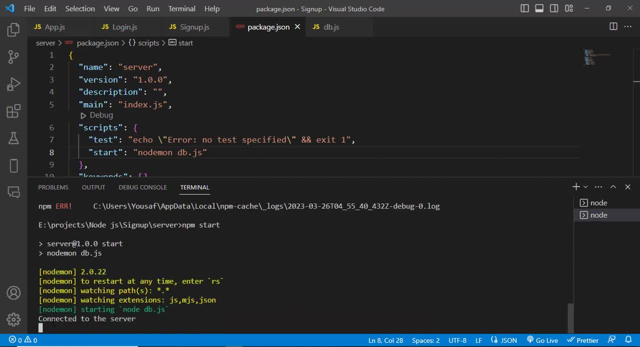 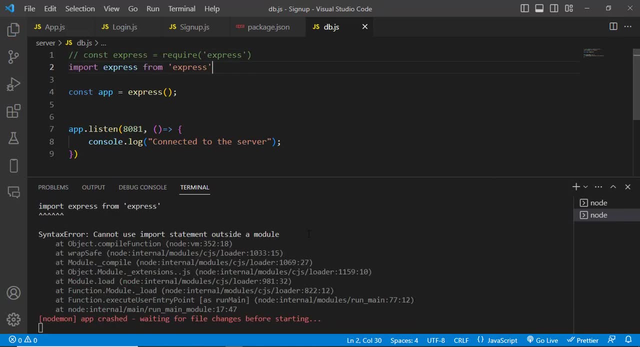 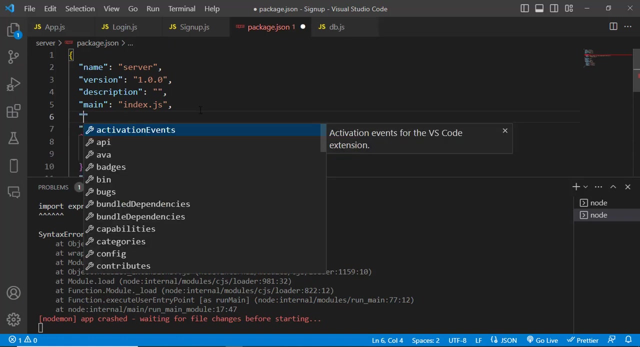 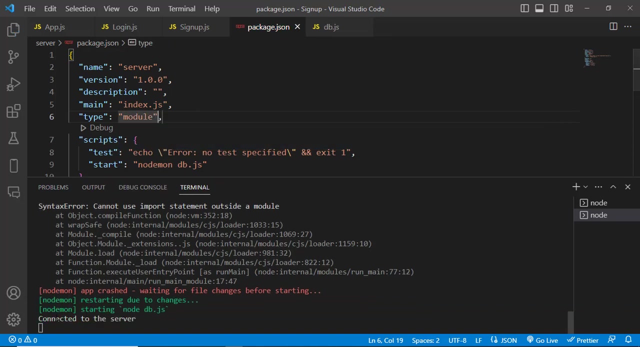 yes, he connected to the server. so now let's come here and just coming down this- and I'm coming, please see, we got in here- cannot import statement so far that we will come here and here we will write: I let's see connected to the server. so that is working, it's fine. let's close this. 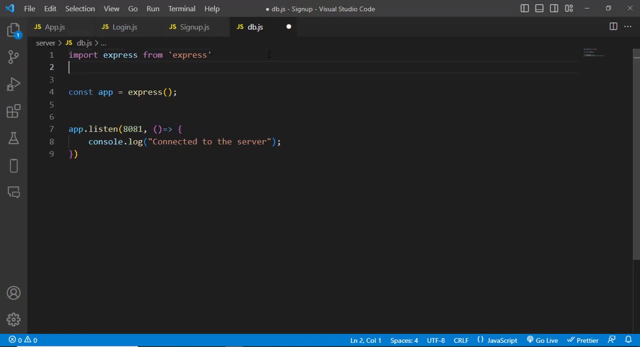 and let's remove this one. let's import the mysql now. import mysql is equal from- sorry- mysql import course from course, and after that let's use our course. half dot use should call that. and also whenever we pass data to this dbjs file, that should be first. 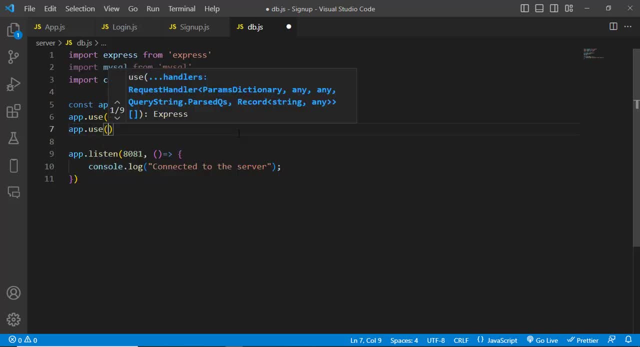 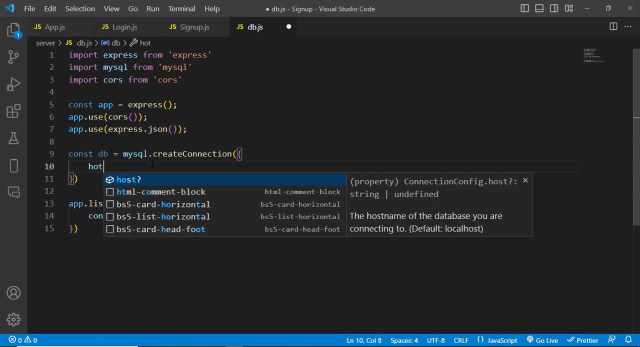 to the json format. so for that we will use of that use i express dot json. yeah, we did the initial things. so let's create connection with the mysql data base. so for that we will like const db is equal to mysql dot. create connection and here we will pass the properties. the properties are: the first property is the host. 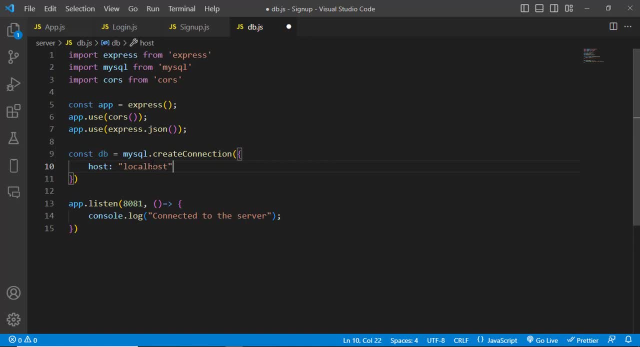 we are working locally, so localhost and in the user, by default, the user with me is root and the password: i didn't set up the password, i will leave it empty. and the database: the database without the sign up. later we saw that. so after creating the connection, so now we will create our apis. okay, so now let's come to the 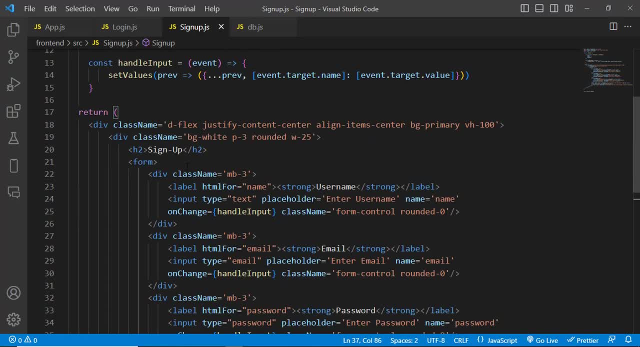 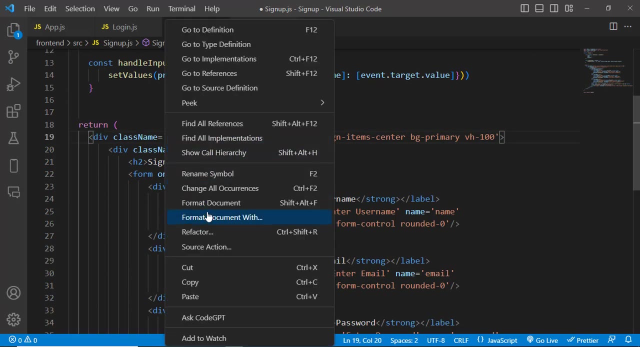 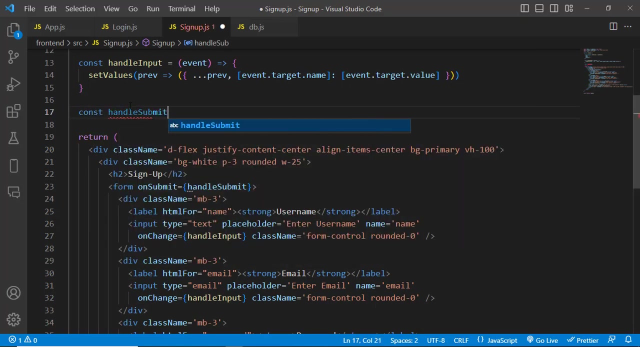 front end to the signup page. so whenever we press the submit button, we will call a function. so let's come here on handle, on submit. we will call handle submit. we will call this function. so let's click that. let's format the document here. const: handle submit is equal to. we will get an event. 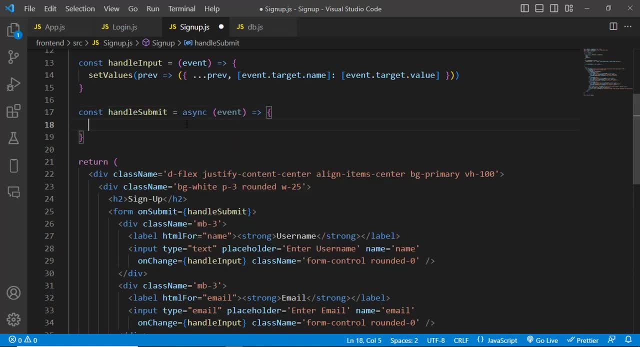 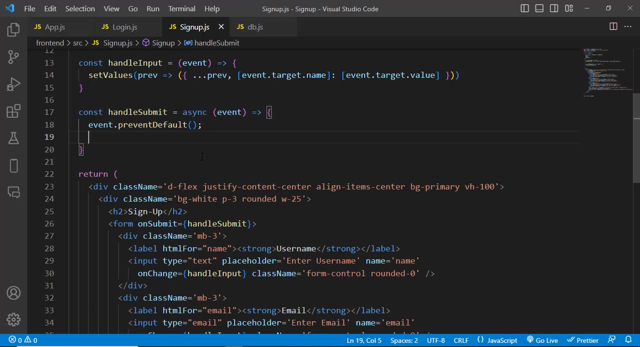 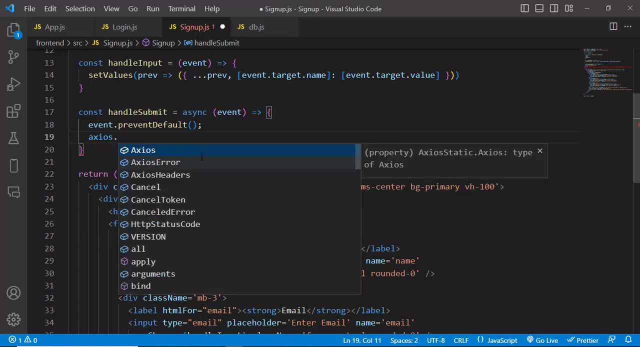 and as it should be the same function with us, so here, first i will like even dot prevent default submission, and after that to far to post the data. we will use access library for that. let's import it, say start. we would like to post the data, okay. 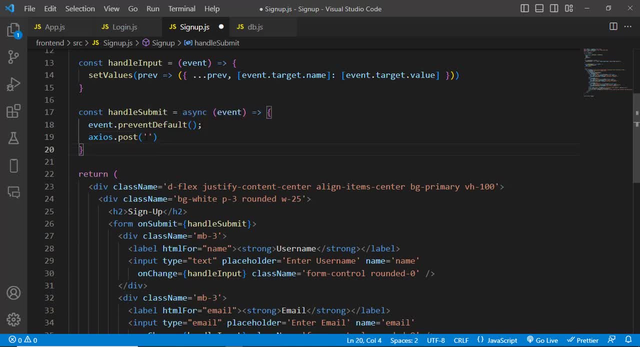 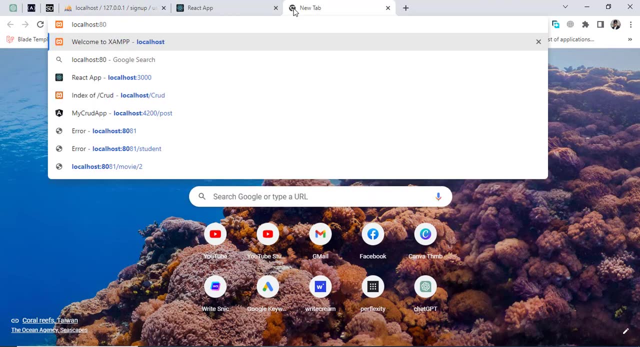 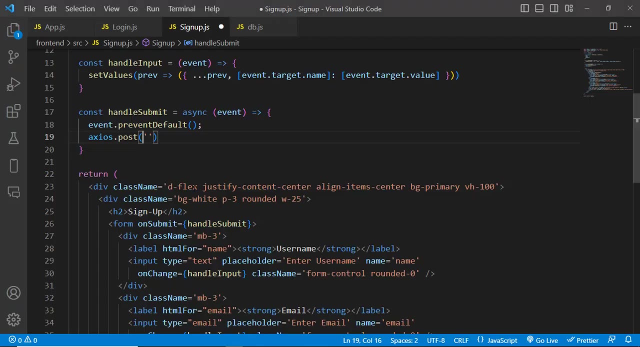 the data for- and here our url- a route that would be: let's come here to local host. our foot server port was 80, 81. let's copy this and we should go to sign up route. sign up, okay. after that we should pass our data with it. the. 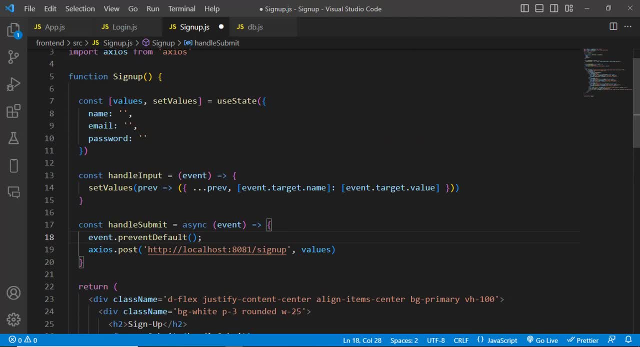 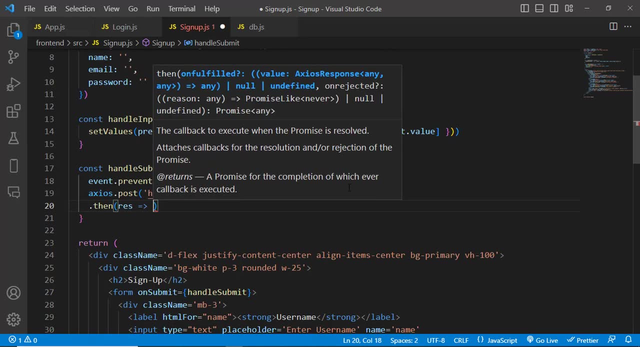 data is the values that we have. okay, this object that we have created, this one. i will pass that now. then we will get our response. if we got a response, so i will just go to back to the home, i will go to the login page. so to go to the login page, i will use use navigate hook from react. 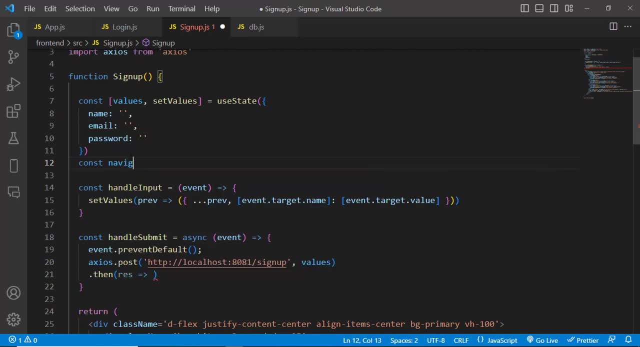 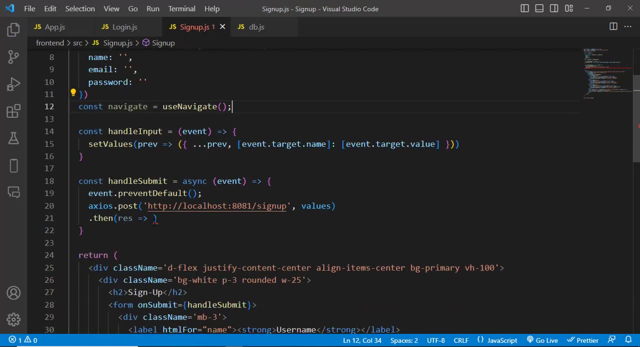 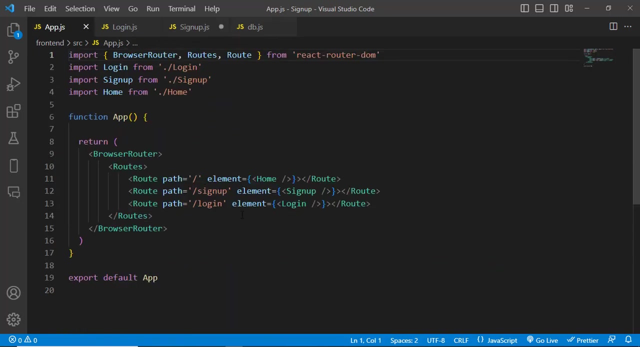 router now. so to use that, let's write const. navigate is equal to use navigate. this is from react router down to navigate to other component. i will like navigate. i will move to this home component. okay, this route we have. we declare this out here. okay, we will go to the home. 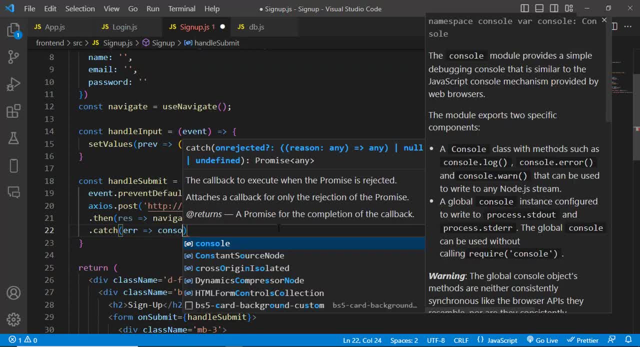 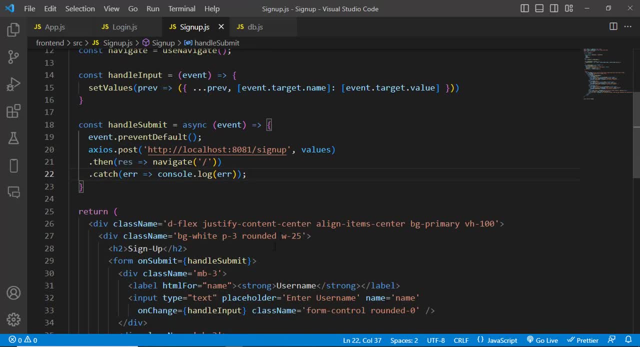 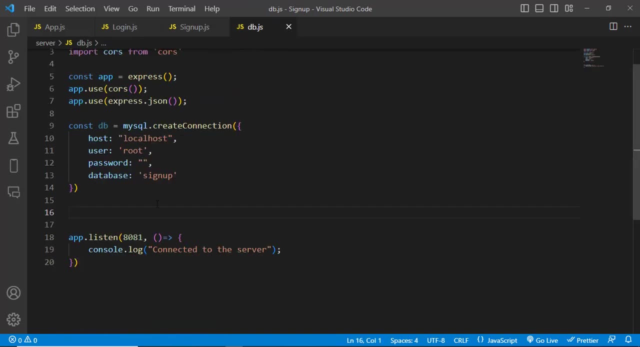 that cage. if there was any error, so console that consolelog here. it's okay, now handle submitted. it will call it. let's come here to the dbjs and inside that we will now create this api. okay, sign up. so let's create that apppost. we will create for the post one. 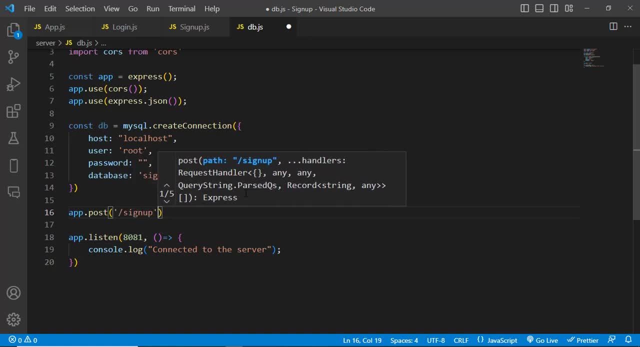 and our route would be: sign up here. we will get a function and we will get a request to parameter request and response inside it. we will let our query now cost is, table is equal to and we will insert insert into that database. the table name was users and we will insert into the name email. 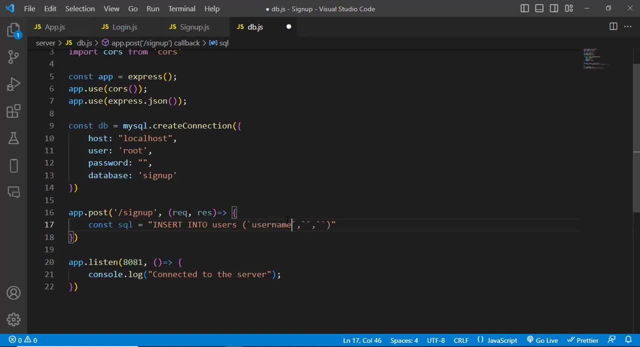 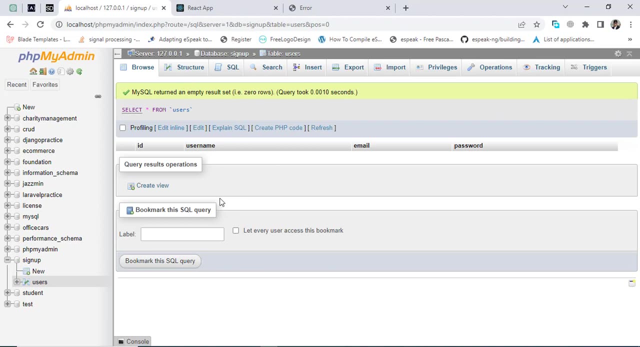 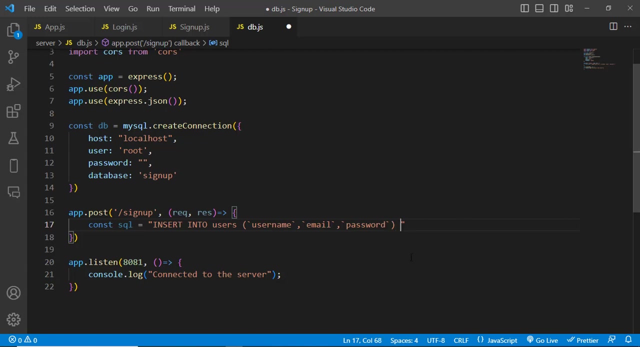 here I should write name, username and email password. let's check our table. yeah, username, email and password come here back, and the values would be: let's pause this time for videos. I will just write the question mark. later I will attach that. so now let's turn our query. 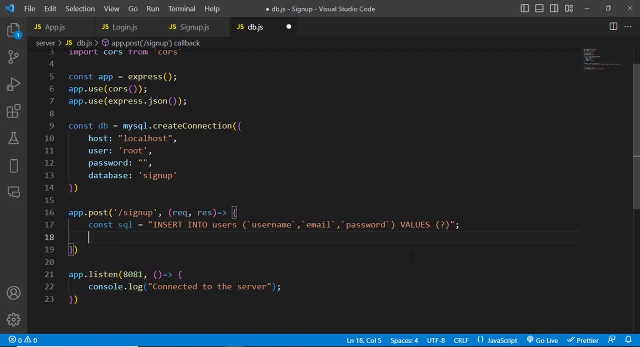 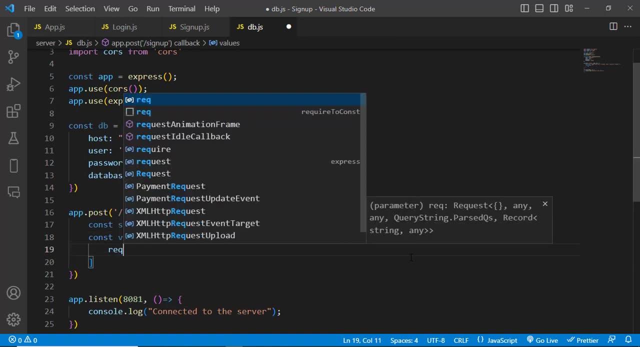 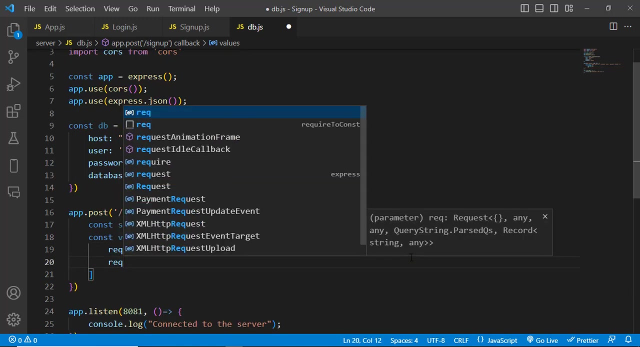 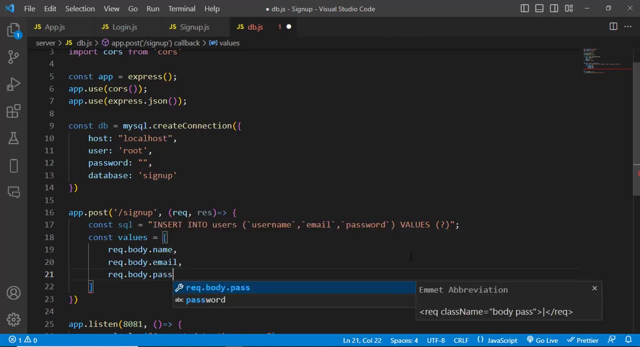 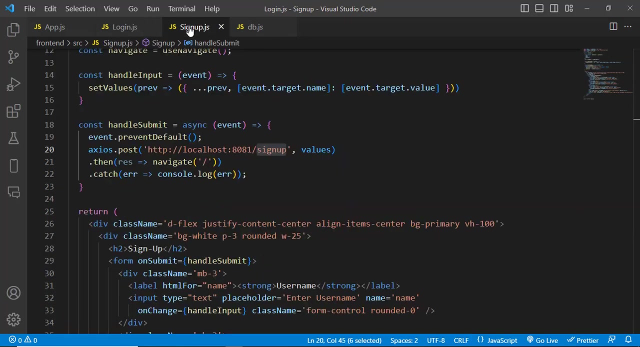 deeper. so first we should get our videos that we pass from front-end. so for that I will like to cost values is equal to in our. a request: that body, that name, first one. in the request that body, that request. start for the password. yeah, let's check that. yeah, name, email and. 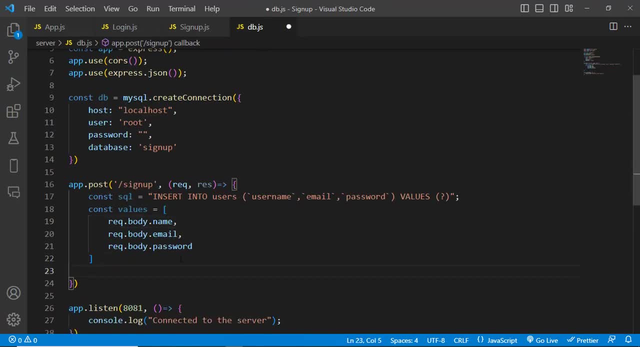 password. after getting that, let's run our query. will I DB object or DB dot very? then first we will pass our estimate, then we would pass our values in a hurry and after that we will get here our callback function. so we will get in error or we will get the result. 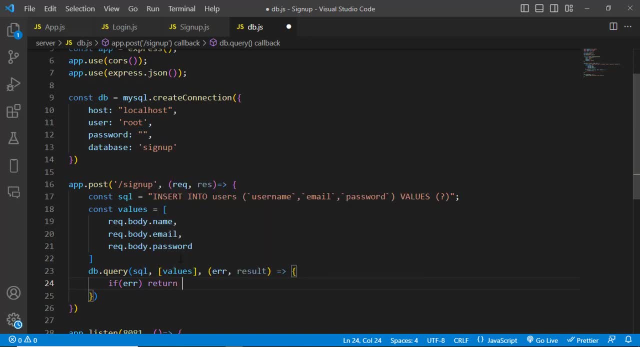 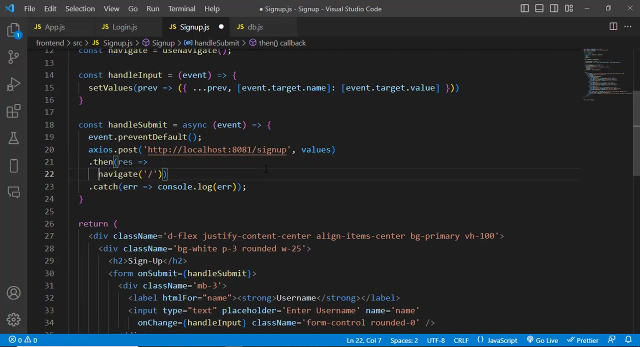 if there was an error, so return resultjson with pass a message here and not yeah, we will just return our result. so let's come back to the sign up here. we will print the result also here. okay, so to print the result, we will first drop it in this. 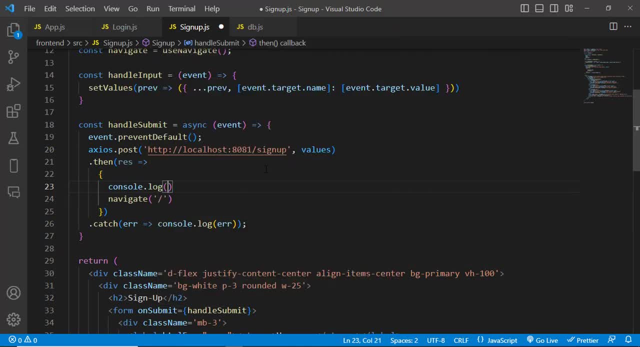 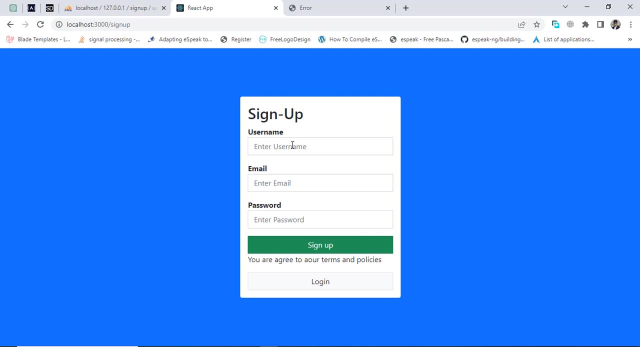 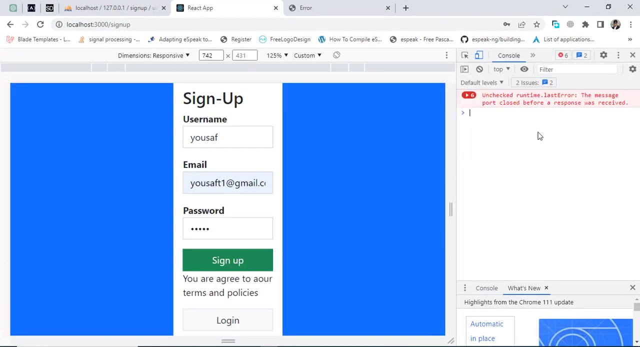 and i will write here: console dot log result. let's come here and compared to the sign up, i will enter a name yourself, t1, and the password would be one, two, three, four, five. let's move to the console. first what we are getting, the result. come to the console, let's press the sign up button. 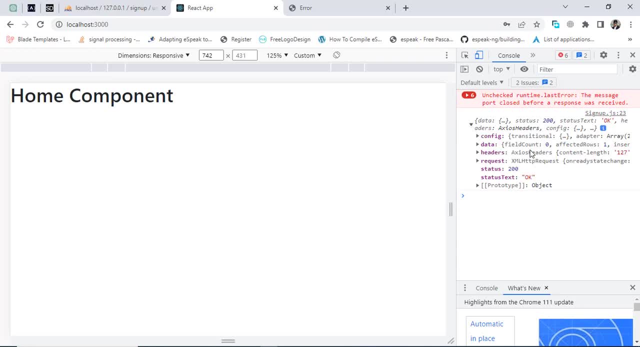 we came directly to the home component and we got the result. this is the result that we got. let's check it. yeah, we got status, okay. and what is in the data side? in the data we have affected rules one: okay, it means that as a record has inserted, okay. so let's check it. yeah, let's check that in the data side. 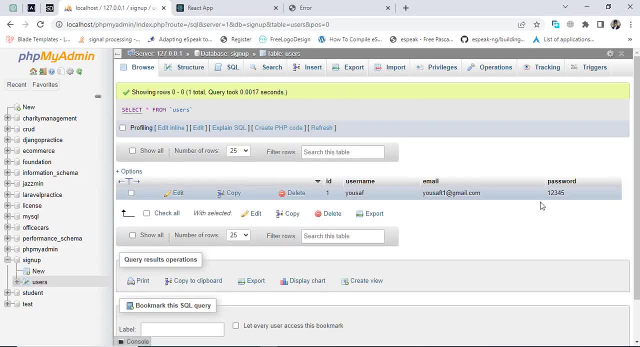 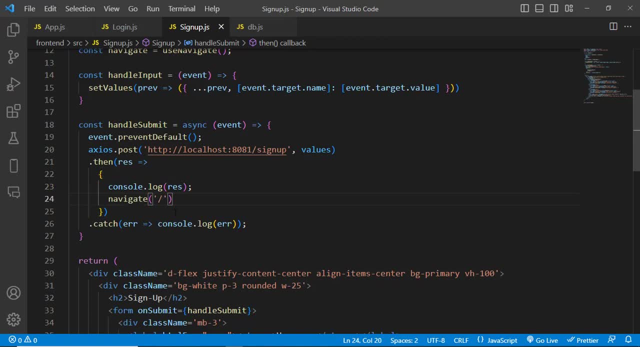 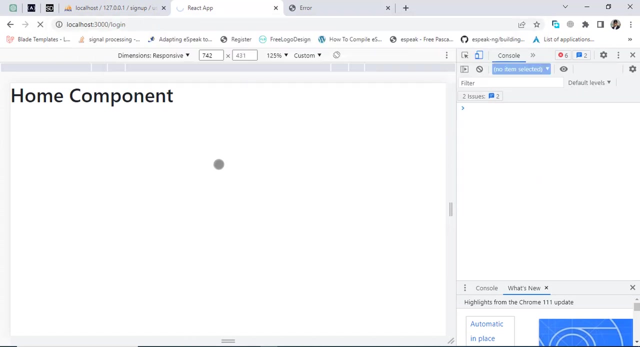 inside the database. let's refresh this. see one. a new record has inserted and we should go back to the login. okay, not to the home component. we should go to the login, so whenever we come to the login page, yeah means we came directly to the login, so then we should write our credentials to log into the page. okay. 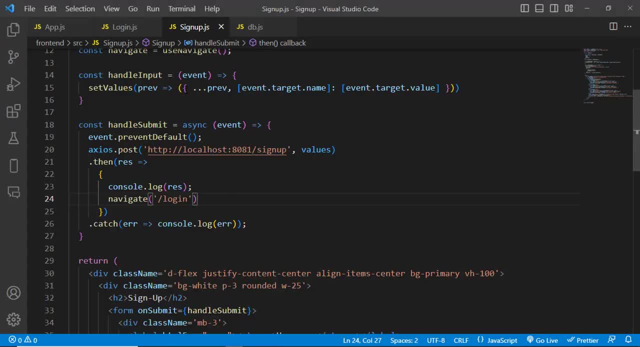 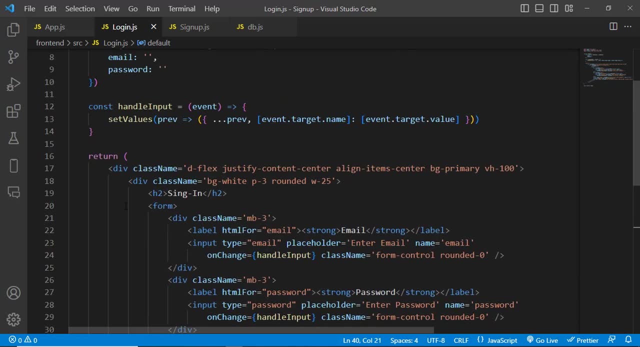 yeah, and we should write our credentials. let's come to the login. so here again we are storing our data in this uh object. let's check them. yeah, here we are storing our videos, email and password. okay, we would like to authorize someone in. authenticate on based on email and. 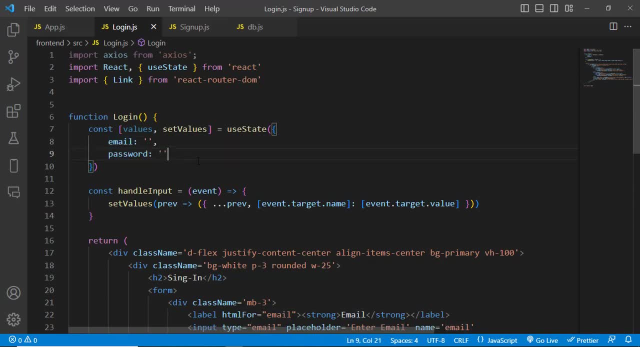 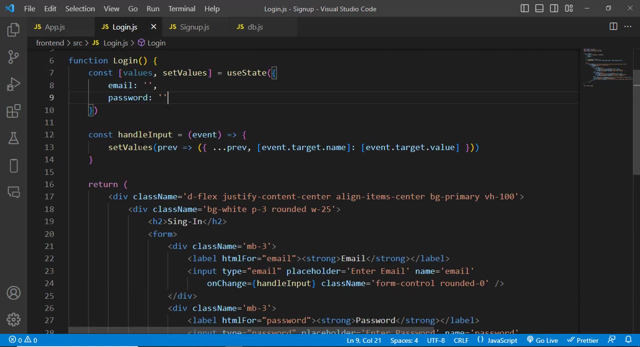 password. so again, whenever we submit here um this submit button, we should call: we should call the login name of our user and then we should click the login name and we should do that. just check that is it valid and not? so for that let's come here, we'll call on. 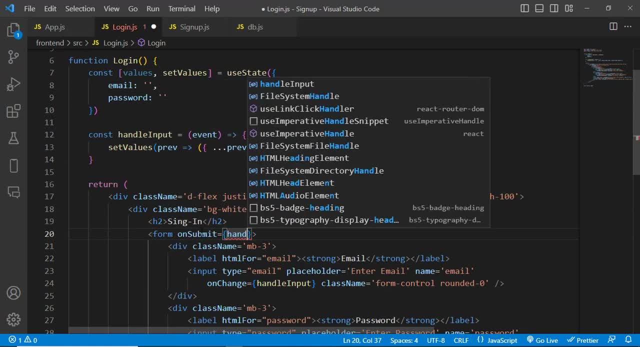 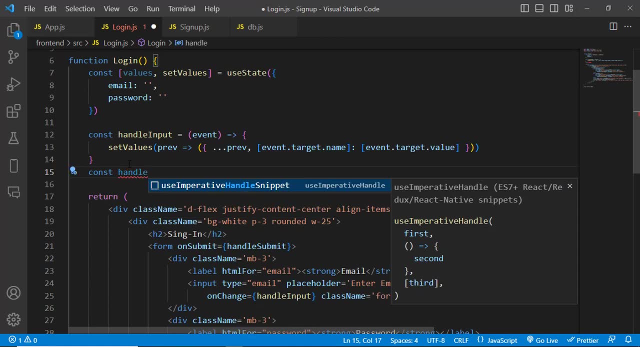 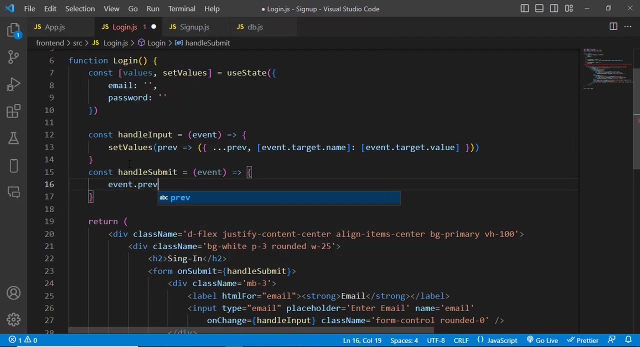 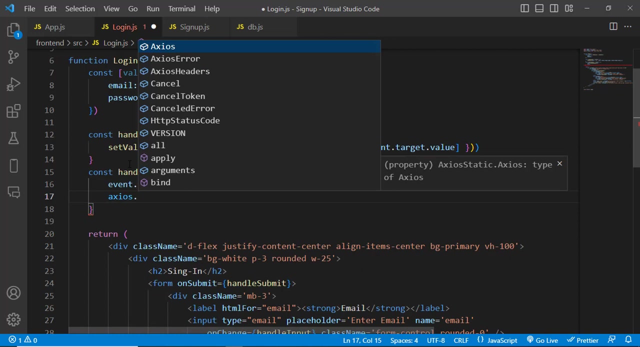 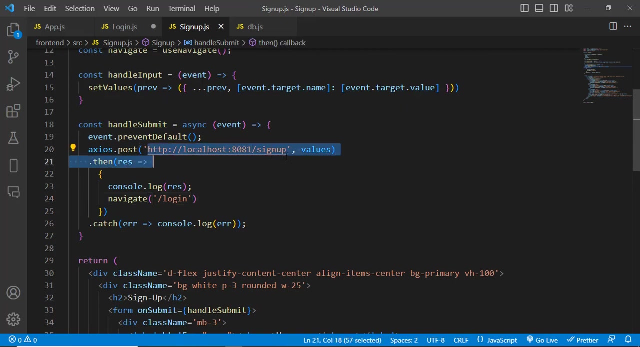 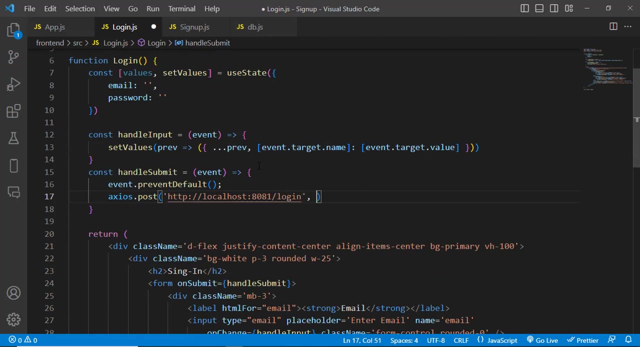 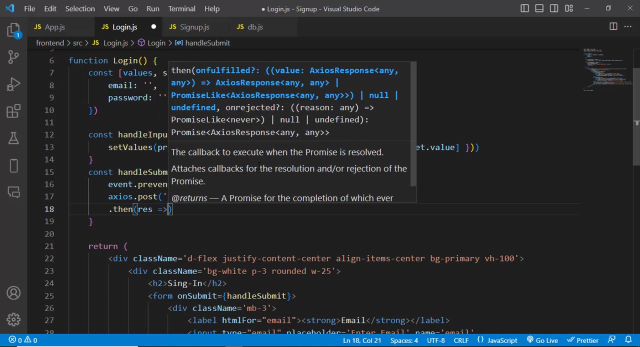 submit, handle, submit. let's create that again here. let's prevent here. we will call again axispost. in this time we should go back to const, handle this route and paste it here. but we should go to login. after login, we should pass our values. by passing again, we will get a result and we will print that. 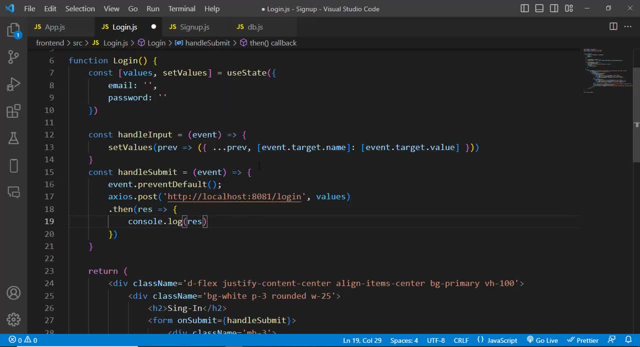 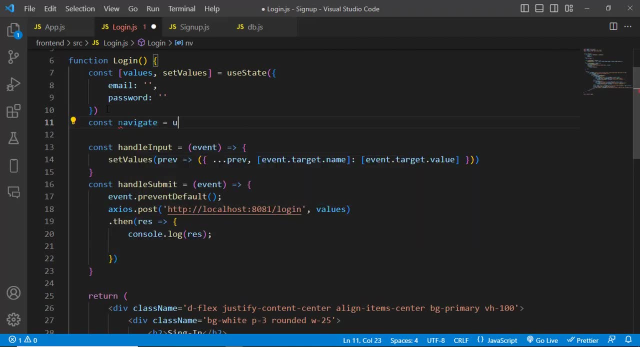 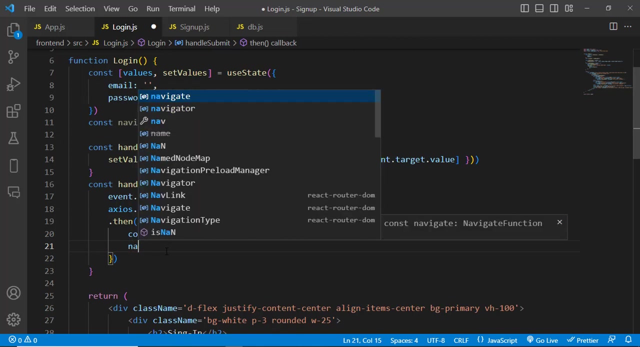 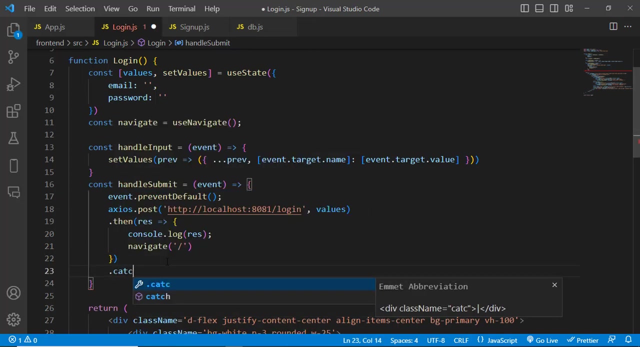 console dot log. and also we should navigate. let's create a navigate object first. navigate is equal to use navigate. and then we should go back to the Home page. dot gage, there was an error console dot log here errors. so now lets move back to our server site. 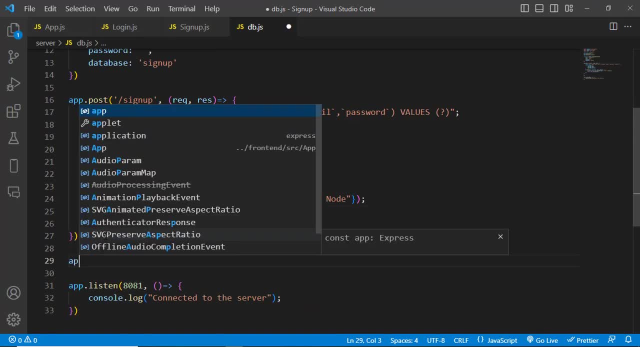 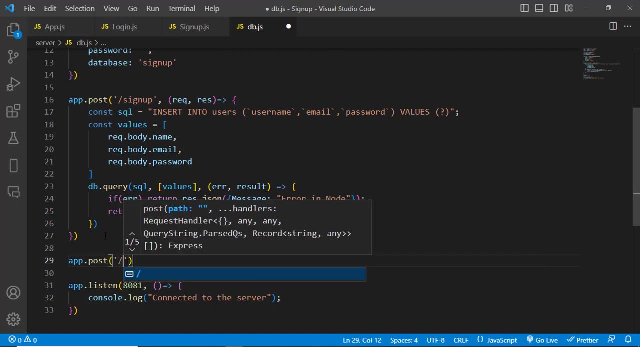 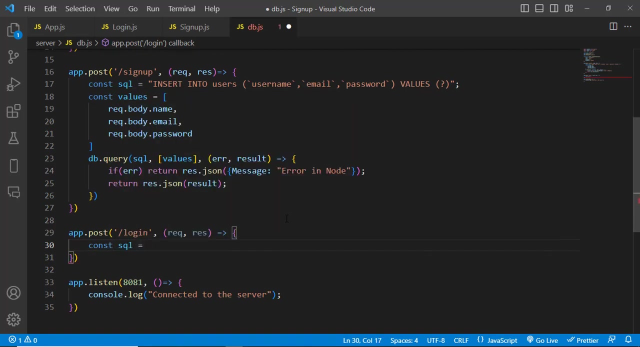 and here we will write an API for our login of that post. again, here we need to request in response and we will write again our query. now we will check that. okay, we will select. select steric from users where where username is equal to with question mark and password is equal to user not. 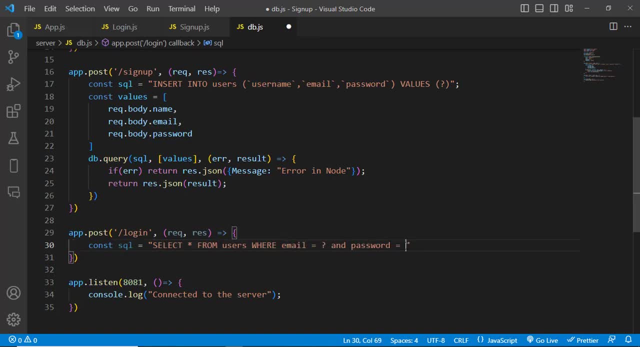 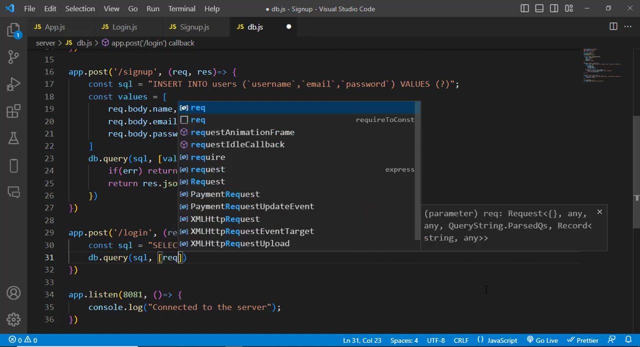 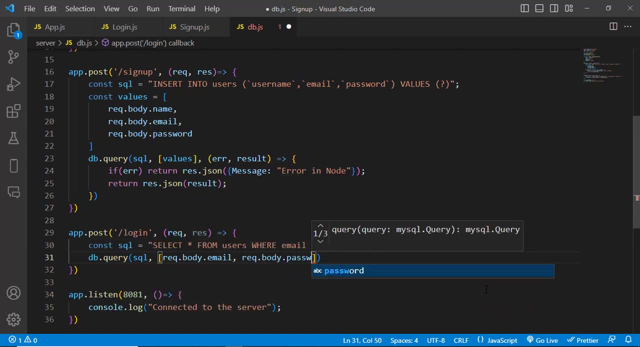 email and also the password is equal to with question mark. okay, so now let's write here: first we will get our. yeah, we will directly run our query dbquery. first write our SQL query, then we will just try to request our body dot email and request dot body dot password. after that we will get an error. our result: 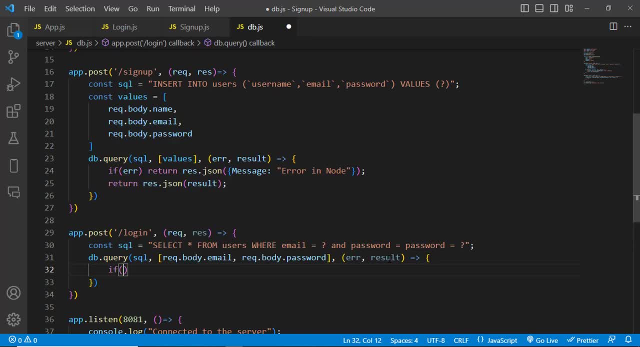 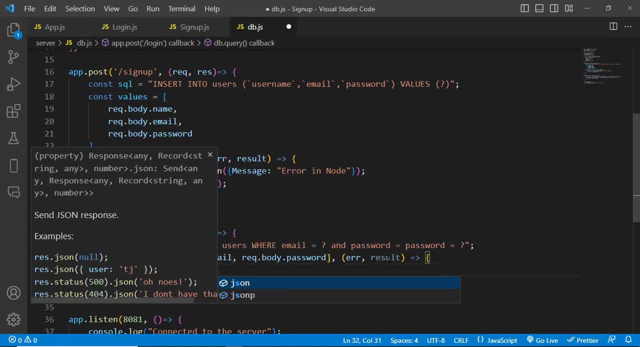 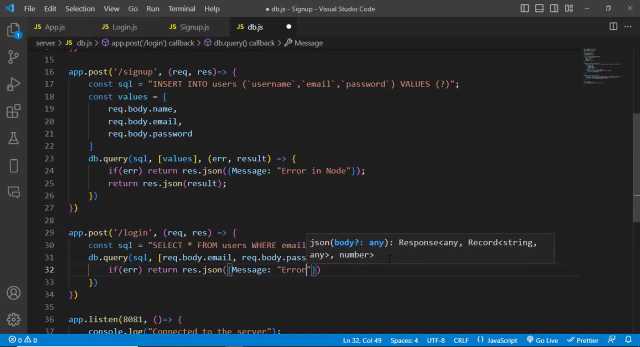 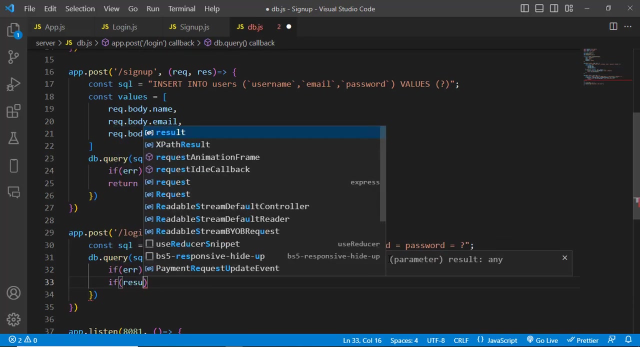 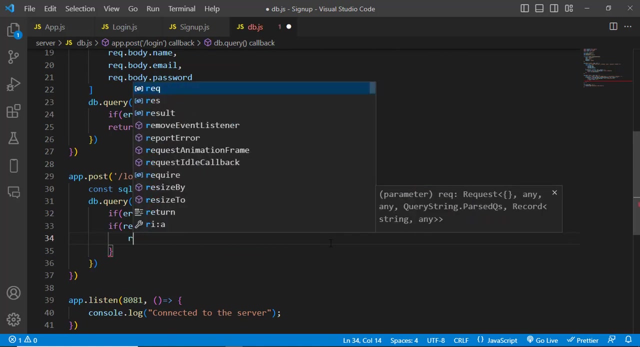 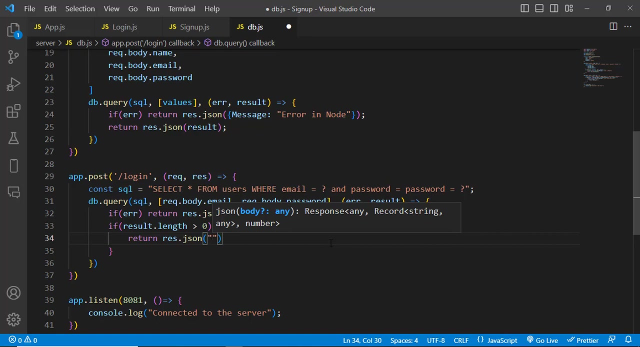 let's run that. if we got an error, so we should return dslr Carson. is we return? no, we will check out the result info. the result that layer was greater than zero, which means there were a record was existed. so we will return result. return is false. 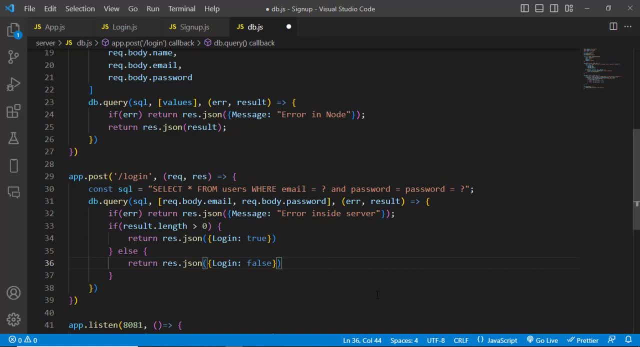 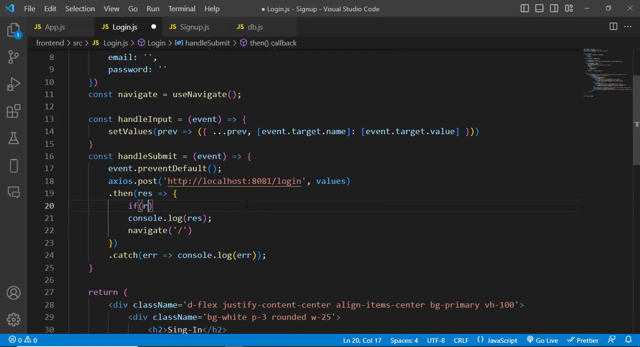 or we can return a message. so let's check it now. let's come back to the login here. we will check if result dot data dot log in. if it was true, so then we should. goes to home page. there is even display a message alert: no record. 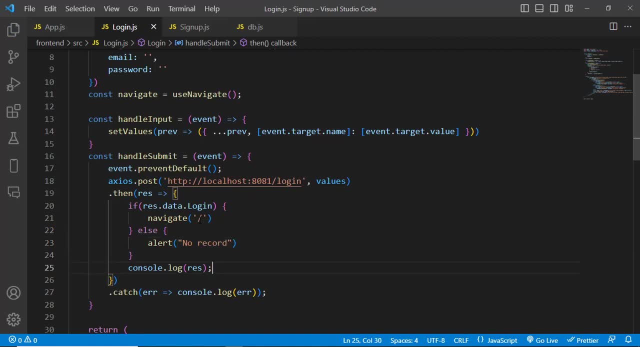 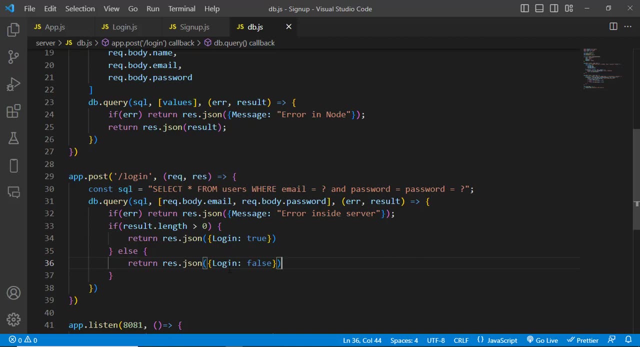 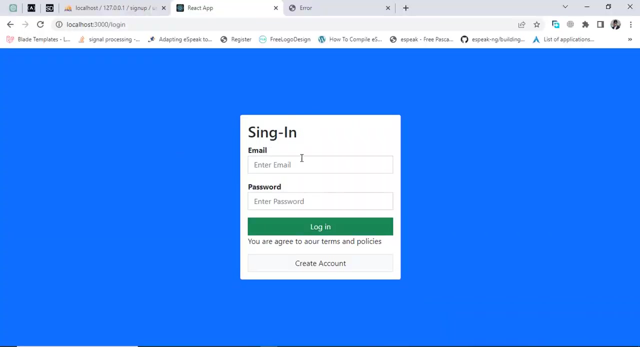 so now let's check it. now let's come here to the login, and here I will like to. first I will like to run email. I will just remove this one from that. right, let's place the login. see, no record existed again. okay, let's add this. 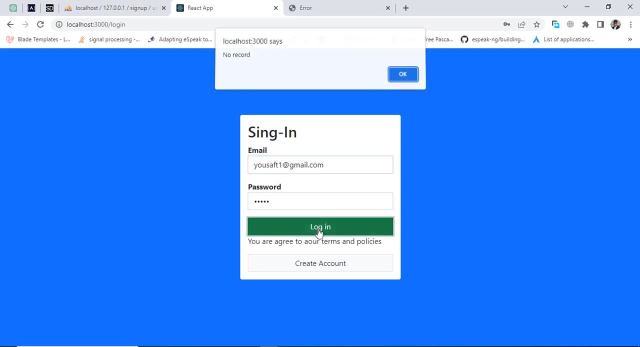 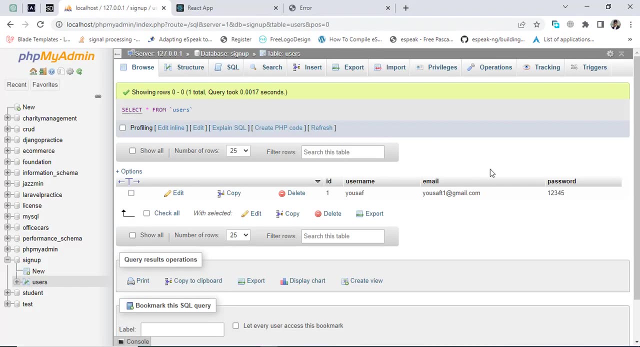 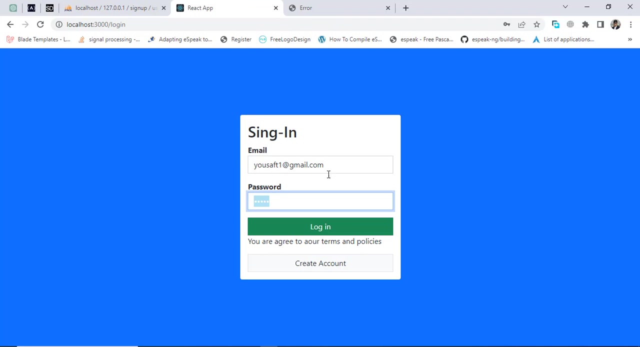 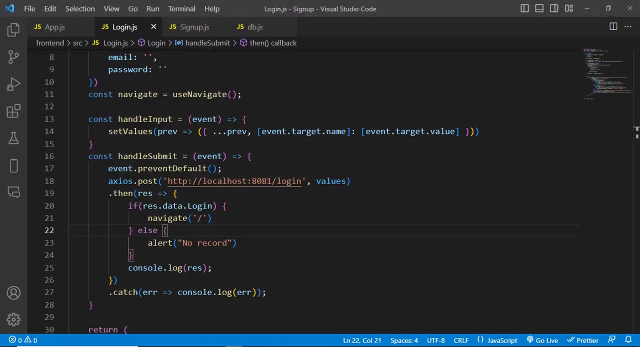 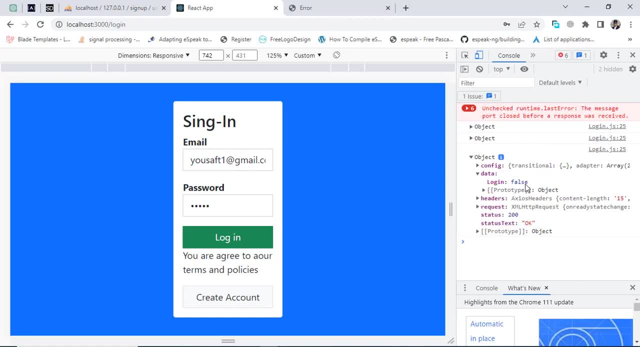 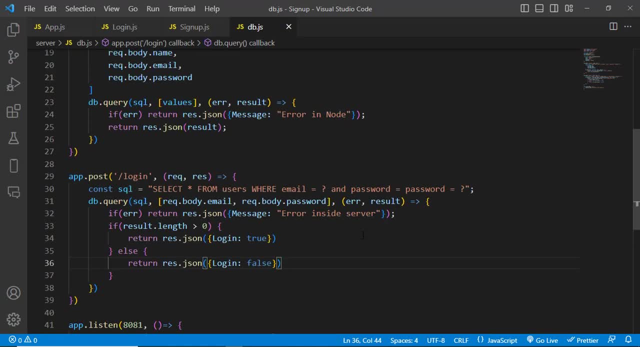 we got an object in the data we have the light in right now. that is false. why? let's come here to the DB dot JSON. so we have written our query. here is the mistake that we were rated twice. the password next. get now and see if it will sí o pause the answer. i think the password. fault. let's check it now again. see, we will return. now. this is our access and hotloast and password. so we have returned. коммент us the password now. so we want to check window. let s the record as well. we can give the password and now we will say that it took the new, whether the password is shank some password and password, as I mean this data was done at the time. object: 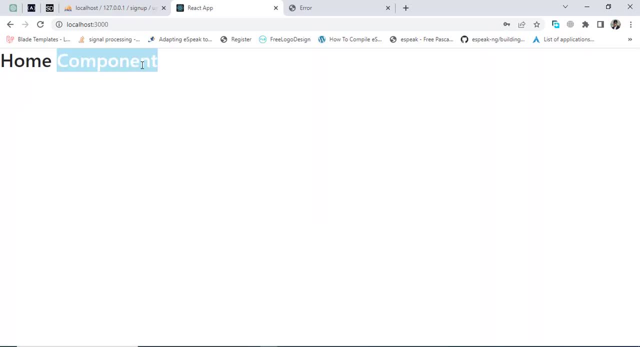 that is correct. that is okay. we came here to the home component, so now let's move to the session and a cookies side, and also then we will check for the authorization whenever someone would like to come here to the home component. if he was authorized means like it, so he should come here, otherwise he should go. 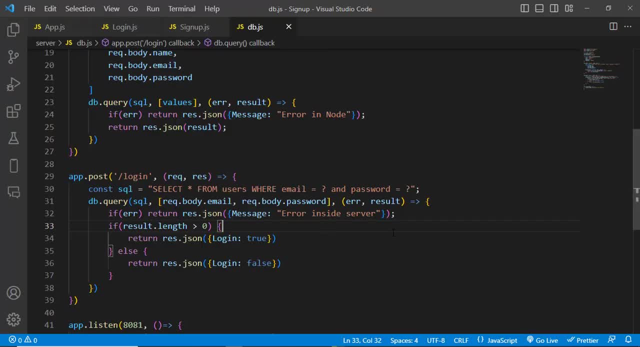 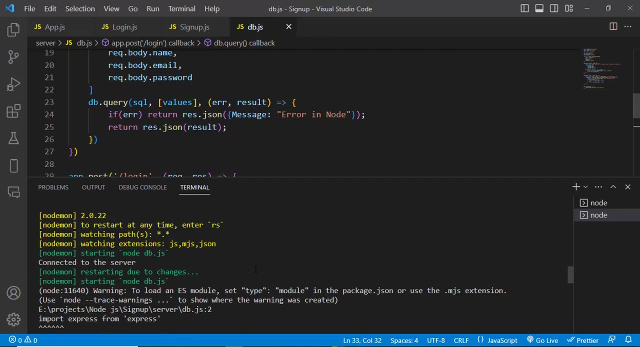 back to the login page. so for that first we should install a few packages. let's go to- or, yes, it is, we are the server side. yeah, here we will just and it's full creation and here I will just need to serve. inside, the type will install. 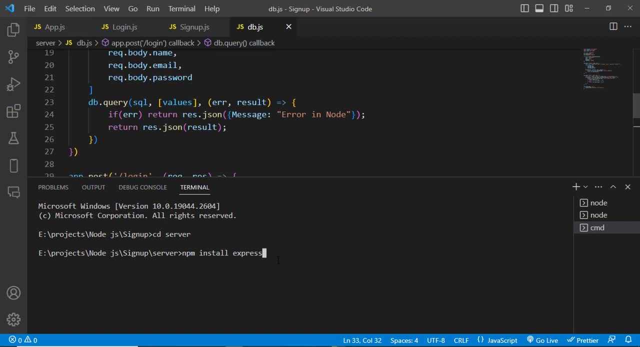 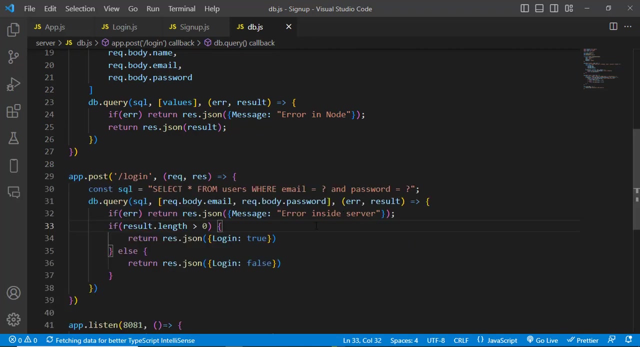 and will install express session and, after that, body for sir and cookie parcel. these are for the session and cookies that we should install. so let's reset and install them. yeah, they are installed. so for installing them. so now let's use them. so let's, first of 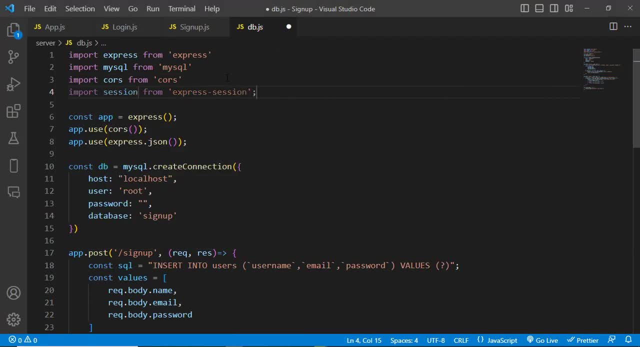 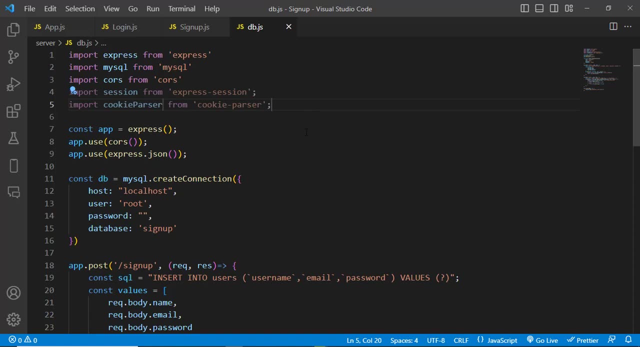 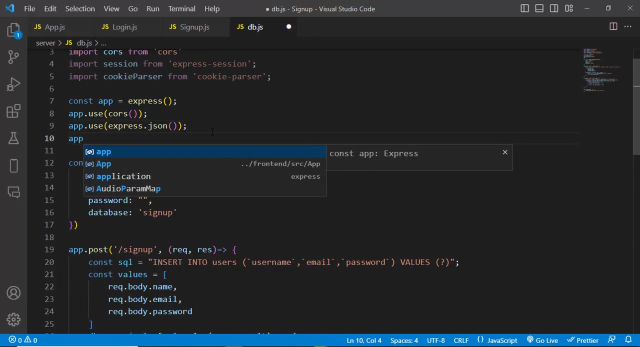 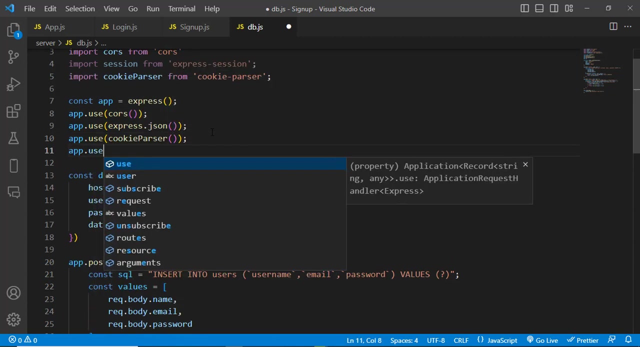 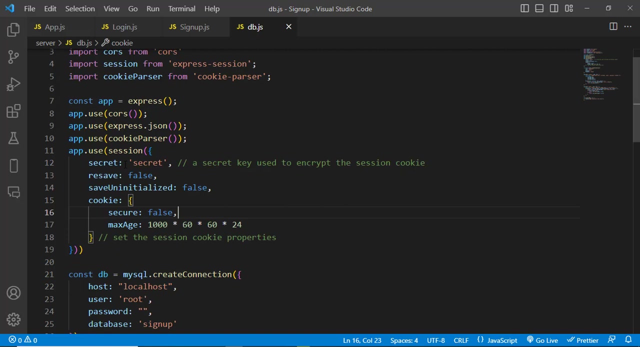 all import them, import session from express session and also import cookie parser from cookie parser after importing them. so now let's use them, let's come here, appuse cookie parser and after that let's use appuse session and inside that we will pass a few properties. so I have added these properties. okay, secret, it is a secret. 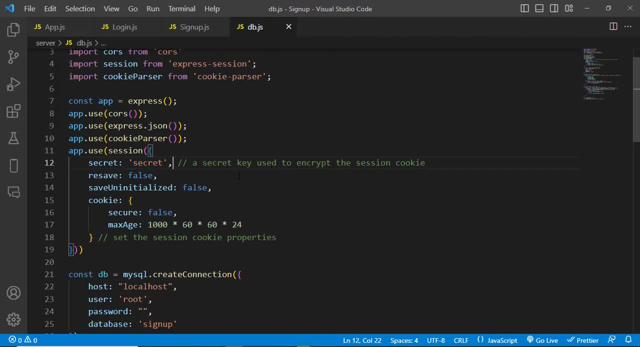 key- okay, which will be used to sign and encrypt the session cookie: receive and then save: uninitialize. this should be false because it will help in performance and to save the storage, because this means that if there is no modification, so it should be false. we should set them both of them to false, okay, and the cookie: the cookie we should. 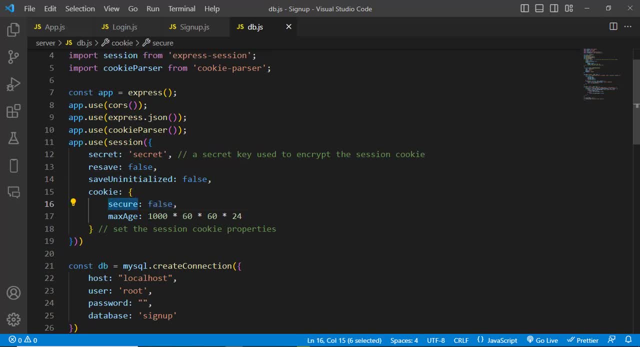 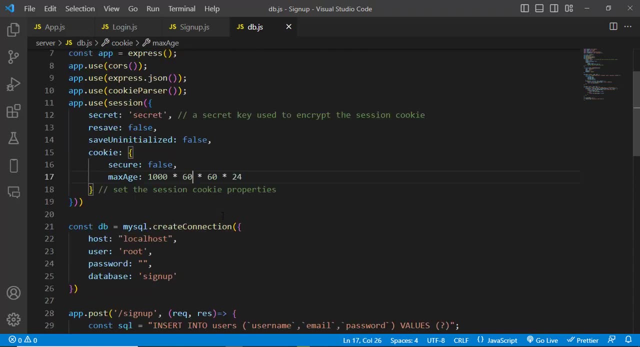 set secure false because we don't use HTTPS right now- and the max edge: it means that it will expire in one day. it is one day millisecond if we multiply it. okay, so now let's come here down to the login. so whenever we login a successfully, so we should set: 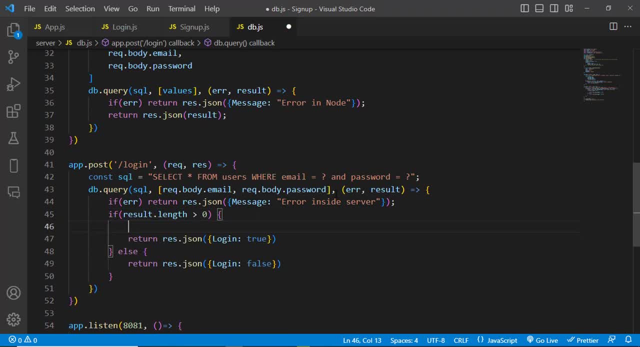 our position here. let's write request session that we will assign username is equal to we will assign. we can assign email also that we got here, okay, and but we will assign the username that would be from result data username. so we assigned username to the session but result is in a rate IP that we should. 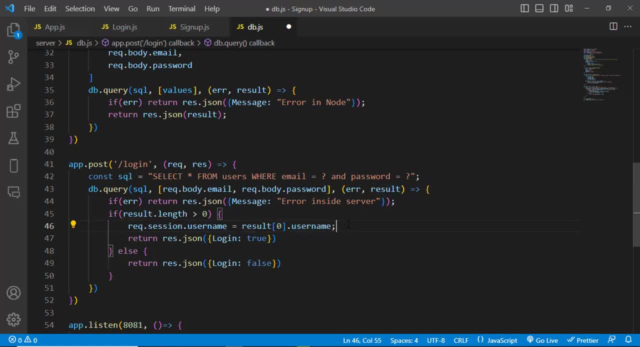 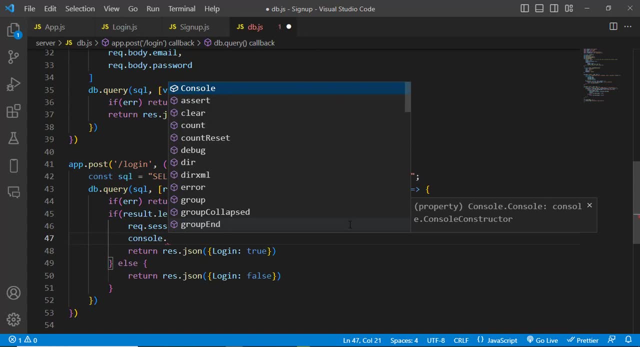 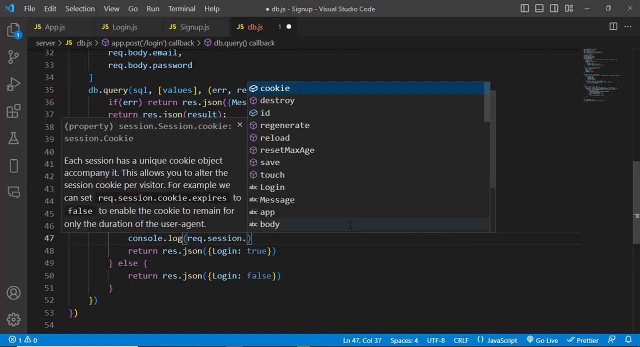 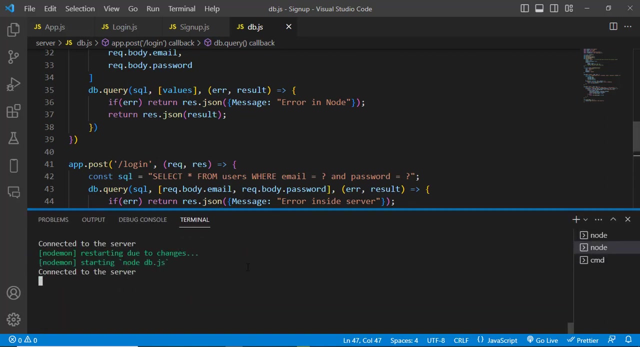 write the first sticker that we are getting. okay, they take the username of that and assign that to the username. so let's first of all check that in the console console, that log, are we getting a request, that session, that username, are we getting it or not? so let's come here and check it here in the server. so let's like it to the. 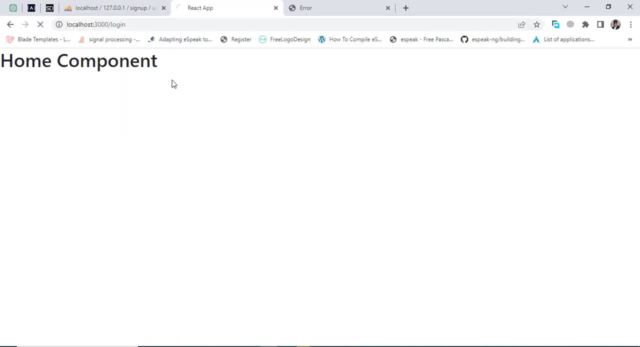 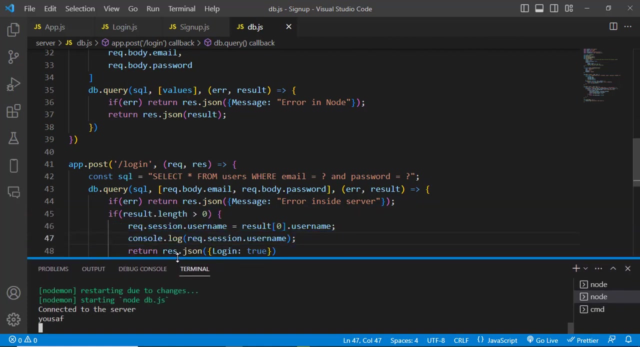 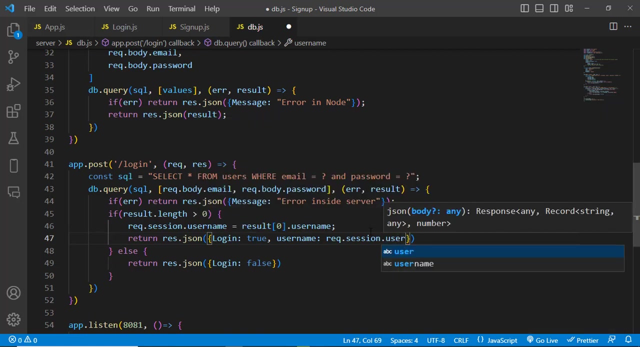 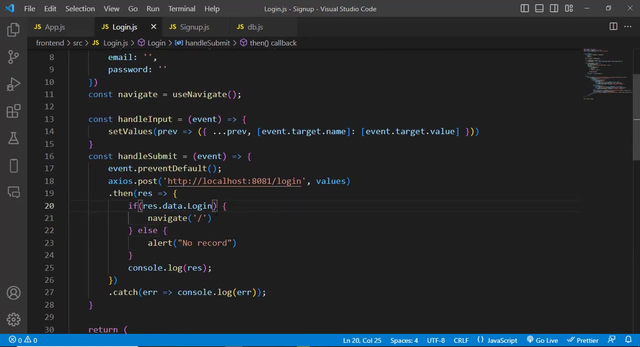 system. yeah, let's check it. yeah, we got our username. okay, it is shit at exit us in our session, so now let's pass our username also here. request that session, that username. let's get it on the login page. okay, whenever we succeeded, so here we should. 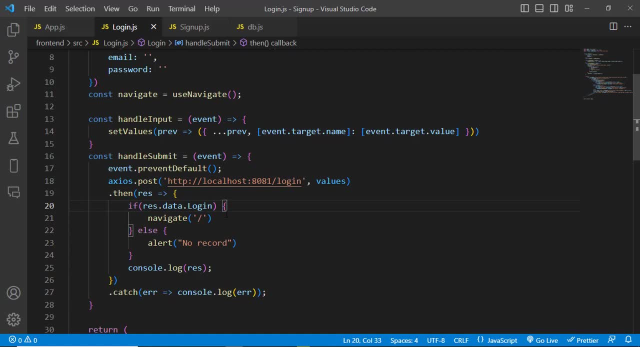 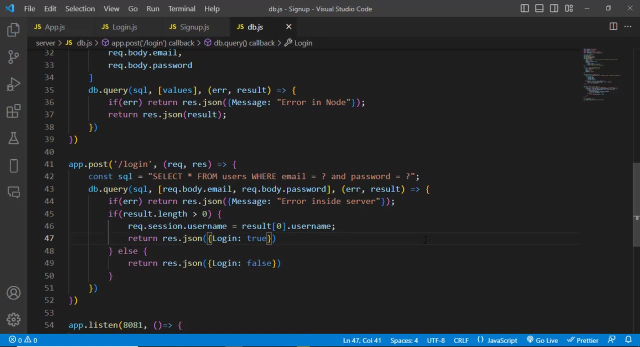 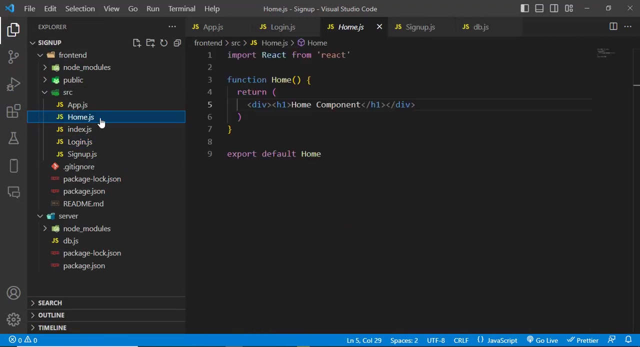 so to access and display that name. we should display that on home page. so let's remove that from this place. we should create a new route. yeah, because we are not, cannot access that here, so let's move to the home component. let's come here and come here to the home component here. we will use that if you were locked. 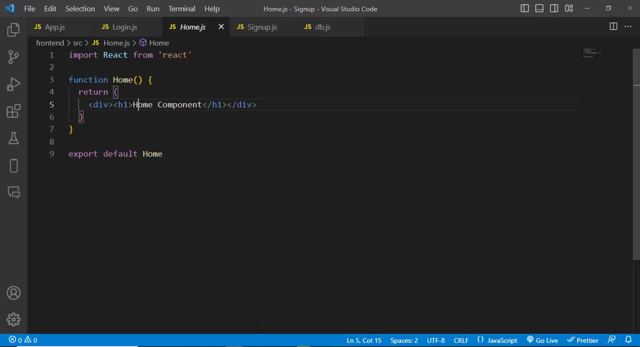 in, so we should display the name, and also if someone would like to access directly the home component. so first we should check that. is this user like in or not? authorization should be checked for that. so let's use. use if it took and we will call a route here. it's any dependency. 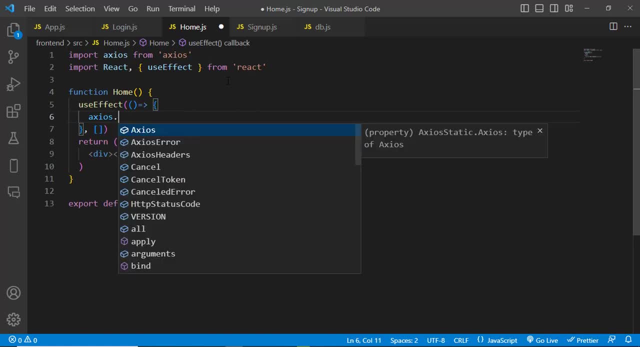 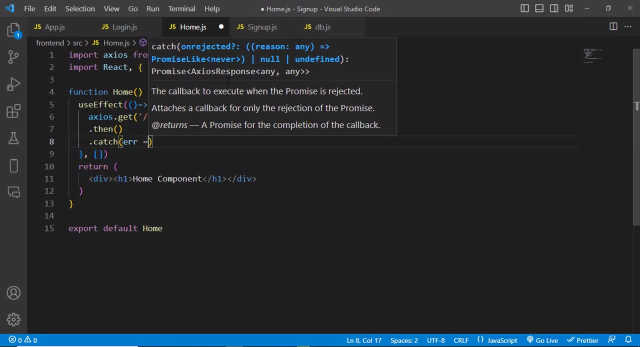 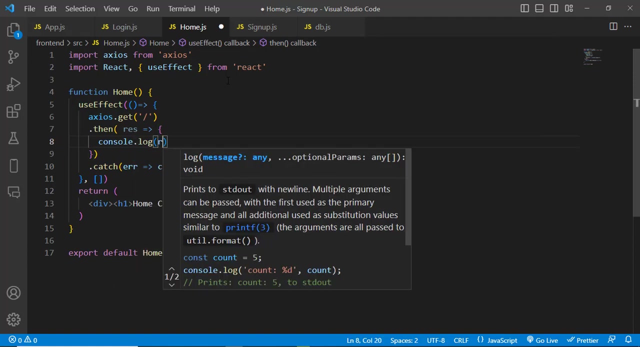 here. so here we will use access library, access dot to a git and here home component, and then we will get a response. if there was an error, console dot, log the air. but here we will get a result and by default first we will console that log the result. let's come here to the DB that is in here we will 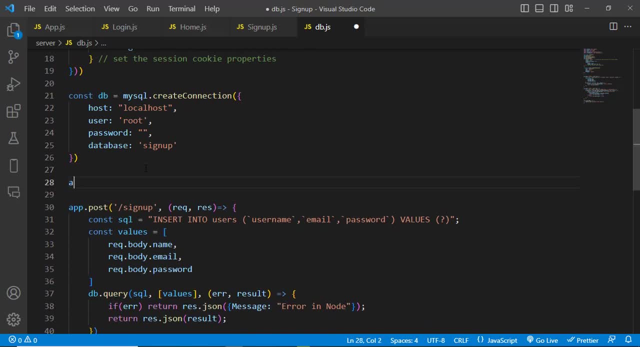 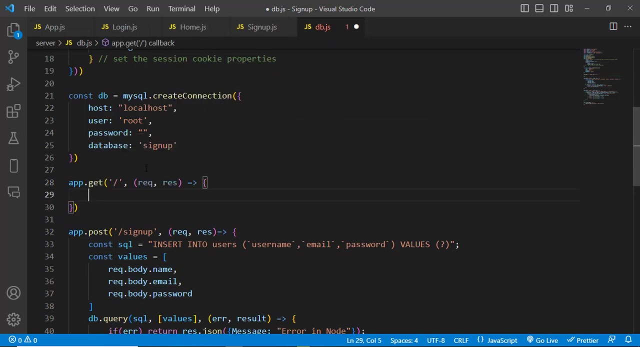 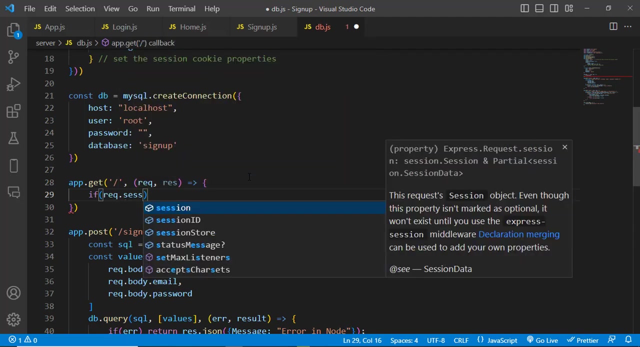 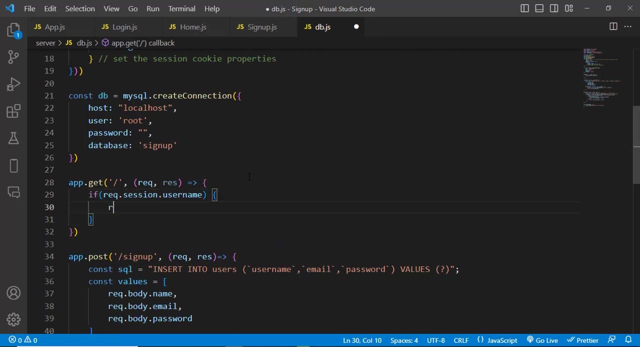 create a new route that would be up that git, that would be home and get that and response, and here we will check if the user was logged in. so we should move to the home component to display the name. let's write a per request: that session, that user name was exists. so then we should just result: return. 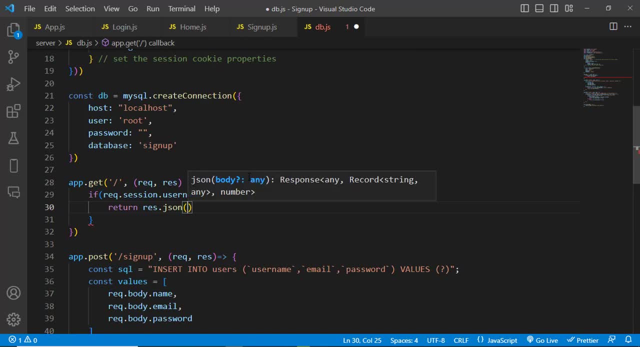 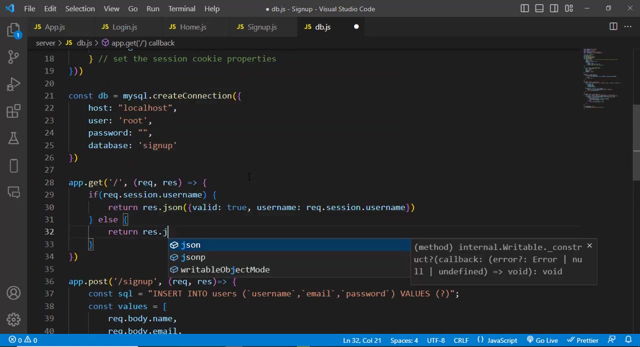 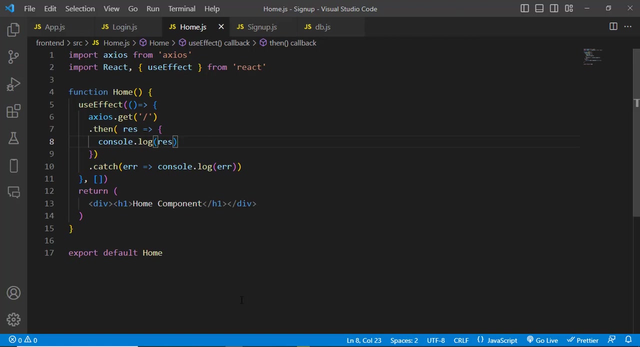 resultjson valid is equal to with true, and also user name: requestsessionuserName. else we should return resultjson valid: false. yeah, so let's move down to the home component. yeah, first we will just display that. okay, we will display that in the console. let's come here, let's move. 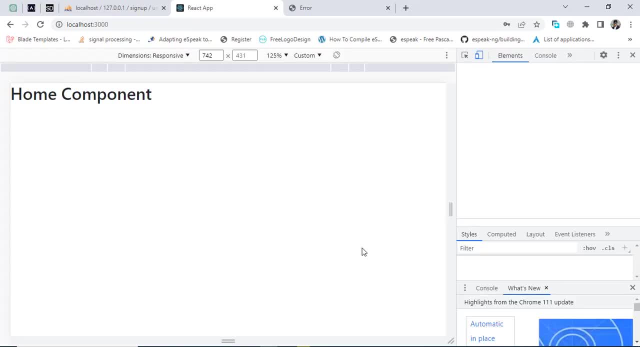 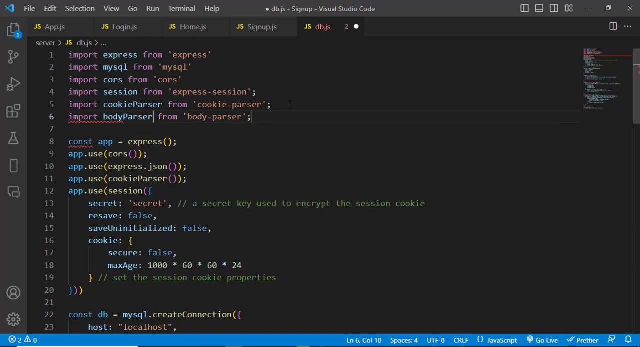 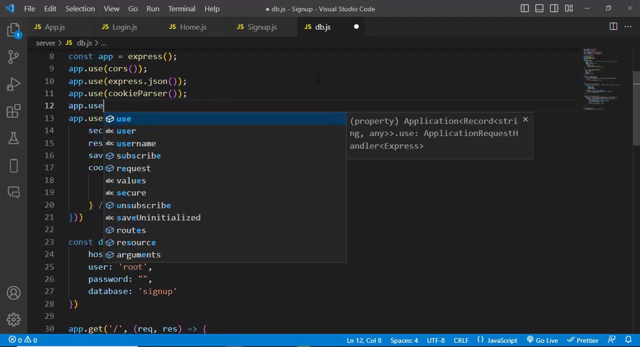 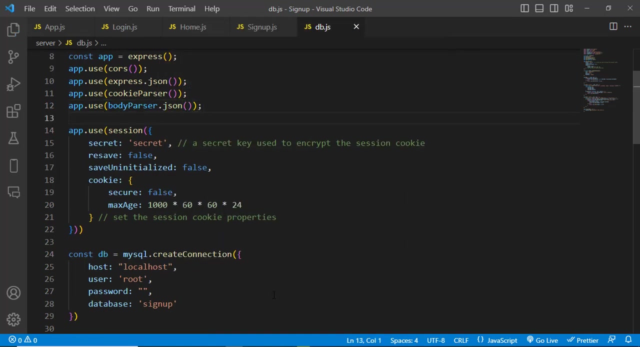 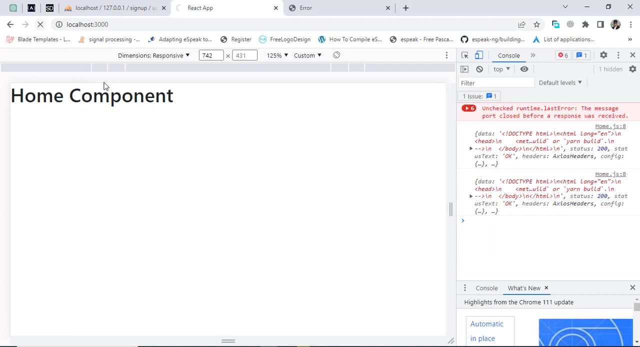 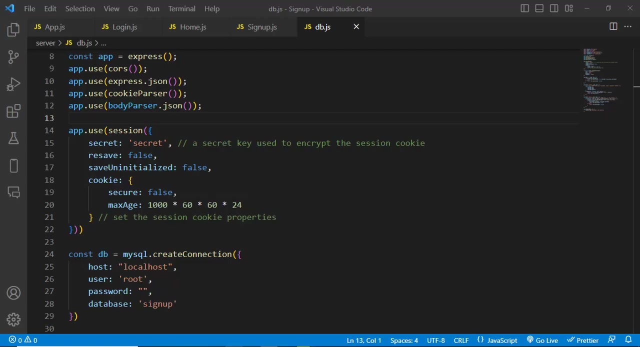 to the console. just come here to the console. we display the name of the user and then we should create the object. we should import body for so, import body for so from body, person, and let's use that, use body for so that, Jason, you, and one thing is that we should use. 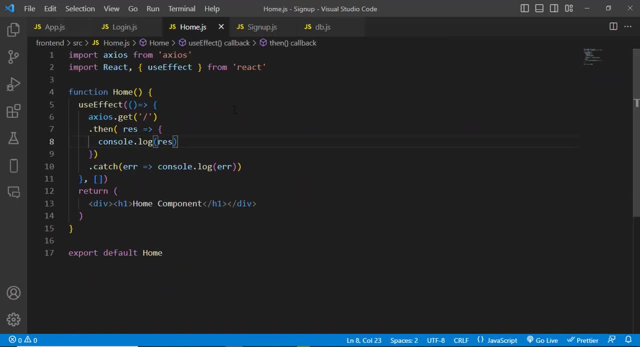 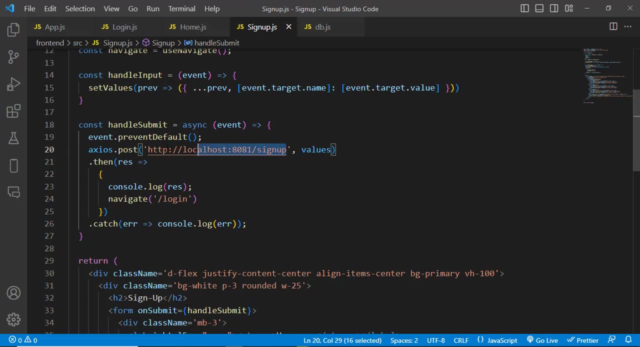 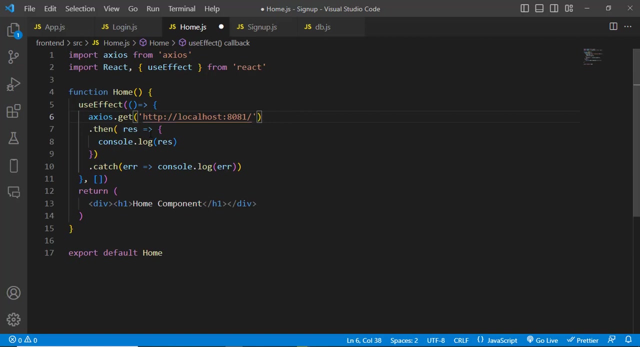 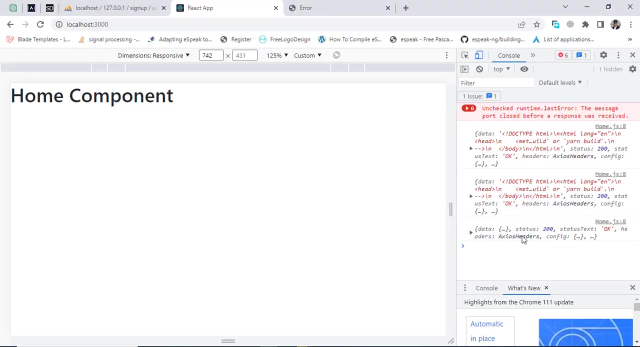 here to the login. oh, we didn't set our path here. sorry, confused. let's copy this and let's come here and let's remove this. okay, we'll move to this server and let's check it now. see, we got this result right now. okay, let's appreciate. yeah, so we got this result. okay, so let's check it in the. 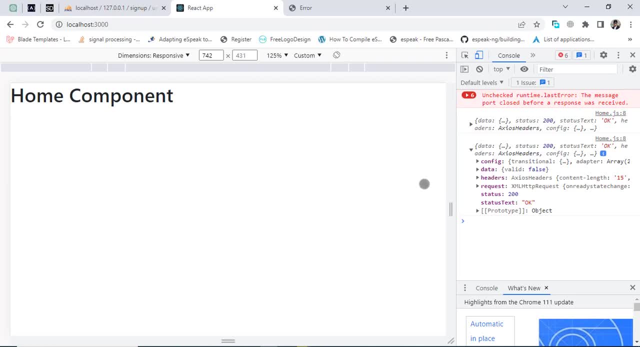 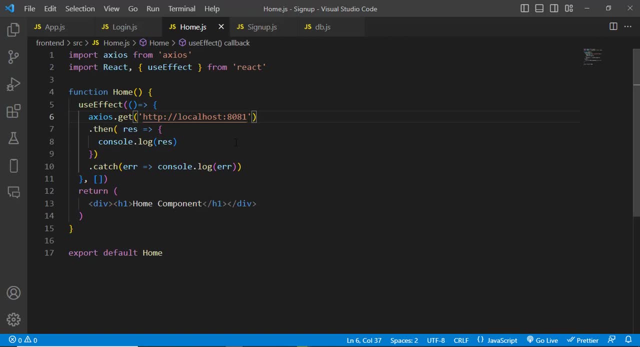 data we got that. well, it falls. okay, it means that the session is not valid. we didn't set that and let's print here: if the session was not valid, so then we should move to the back to the login page. okay, so we will just come here and write result data that valid. if it was true, so then we should. 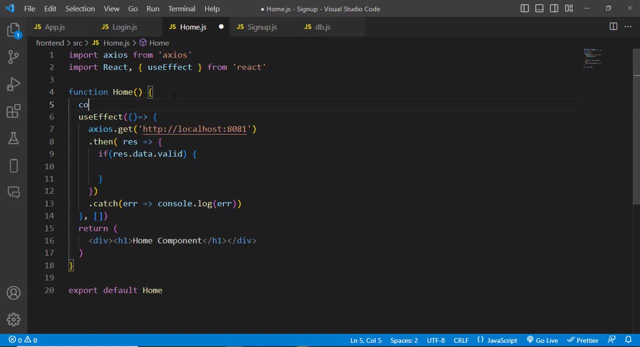 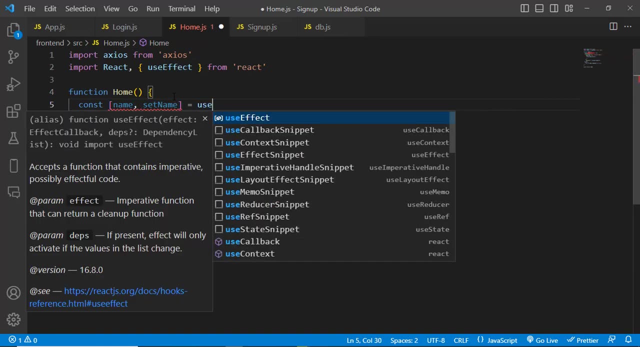 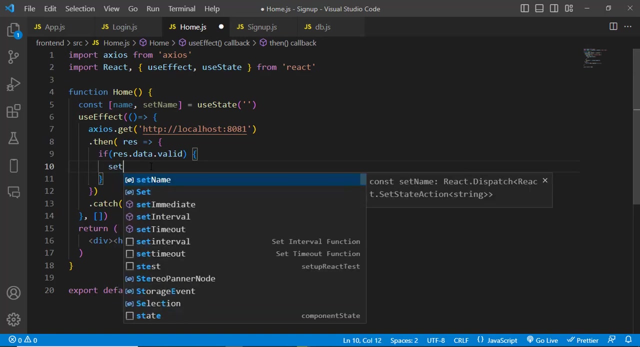 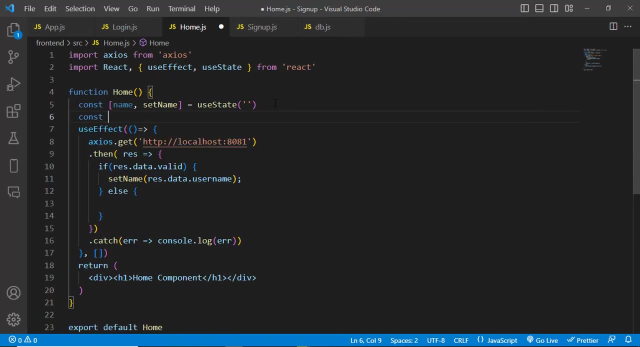 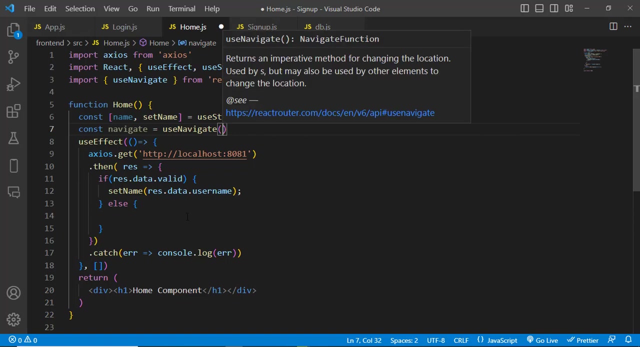 just sit here. we create a variable const name, set name, state hook and we will set our name, set name, resultdatausername that we set. okay, else we will navigate. we will use navigate hook again. const navigate is equal to use navigate and here navigate slash login. we should go back to the login inner, so let's display the name. 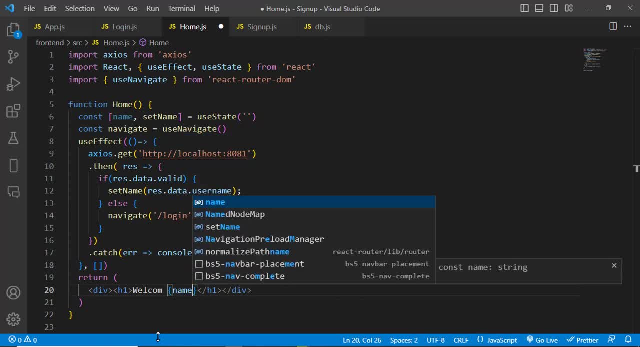 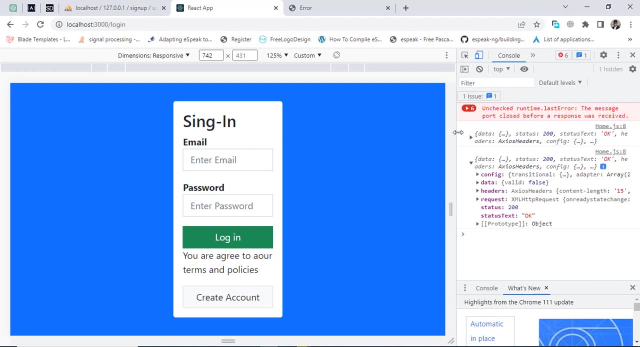 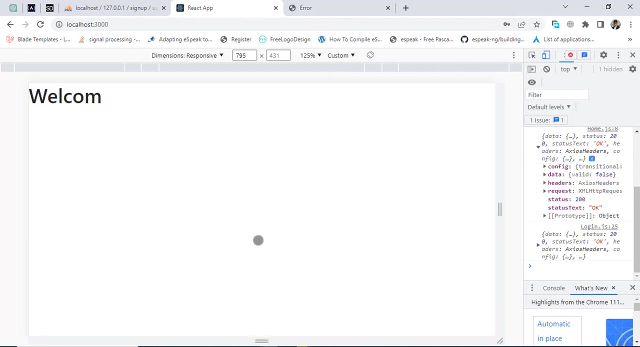 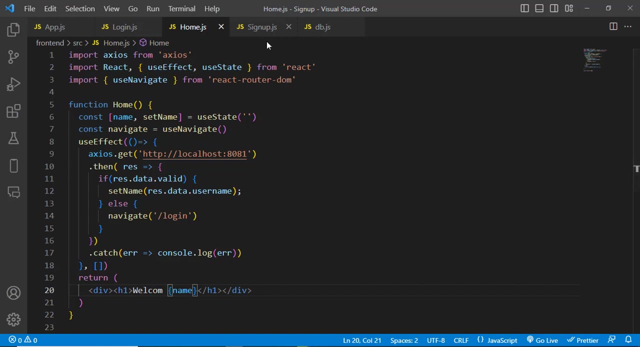 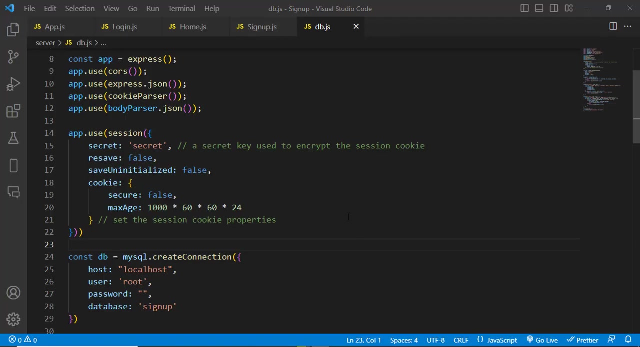 welcome, so let's come here now. so we came back to the login page. okay, so let's log in. yeah, let's place the enter. see, yeah, we came back, but the session is didn't sit. okay, we have problem with our session. come here, yeah, the problem is that we should add here to the course the origin. we should 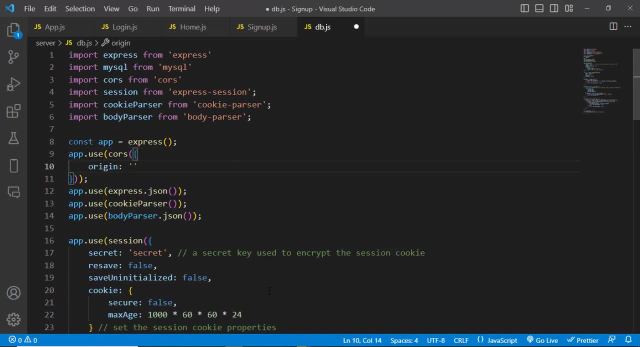 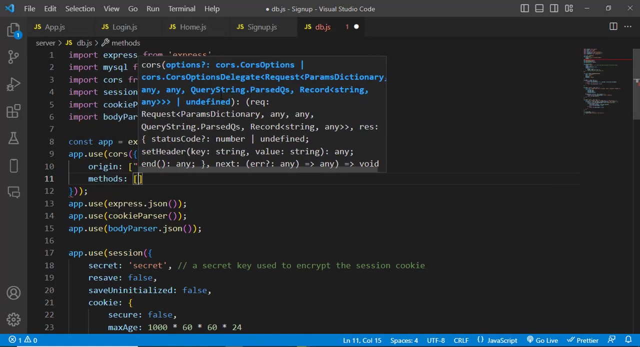 add that here. let's write origin: that is the local host. so let's come here, copy this and paste it. should be in the array. that is the localhost. so let's come here, copy this and paste it to. it should be in the array. let's remove this. this is our origin and the methods that we would like to use. those are: 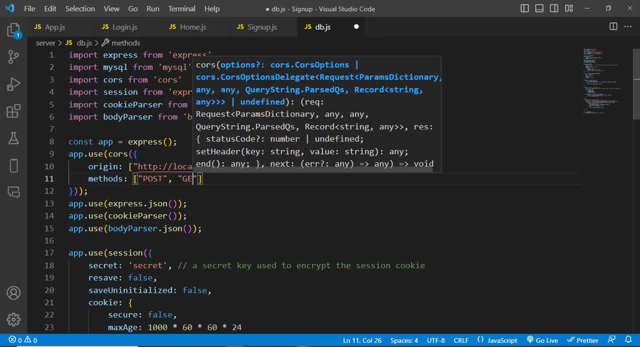 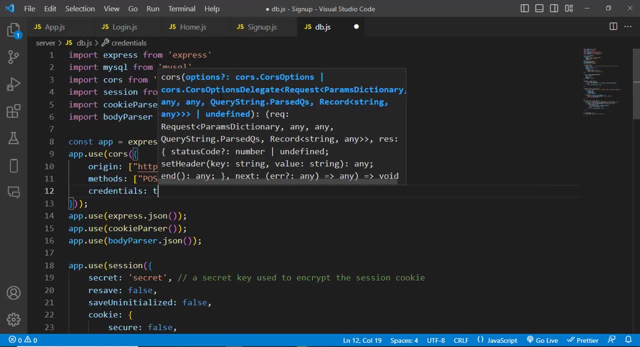 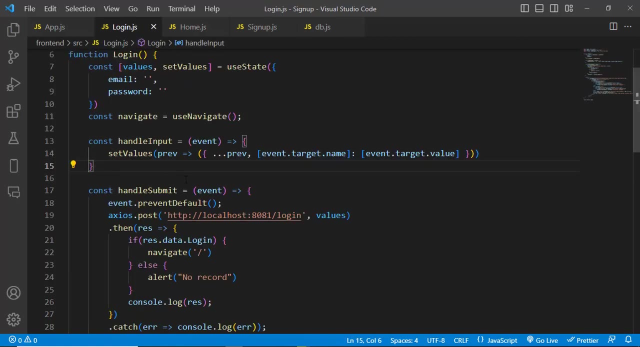 post, indicate method that we are using and also credentials. credentials are true for this. okay, we should specify this, in course, and also we should write here, in the login section: here we should write axis that defaults that with credentials is equal to true. if you don't specify these, it will not work. okay, as we saw previously it was not working, so now let's check. 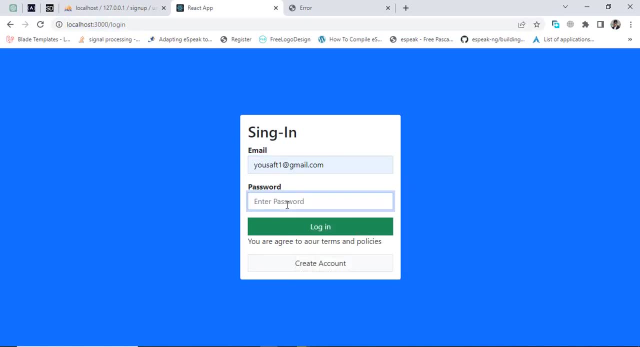 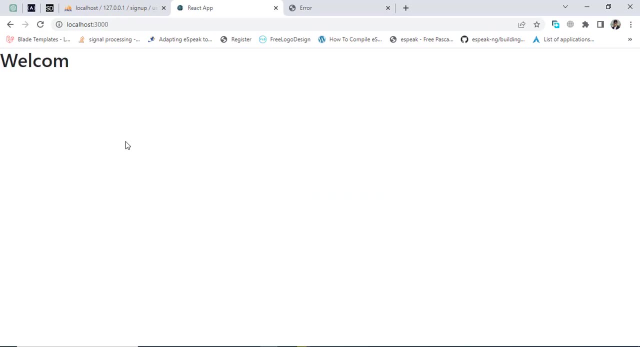 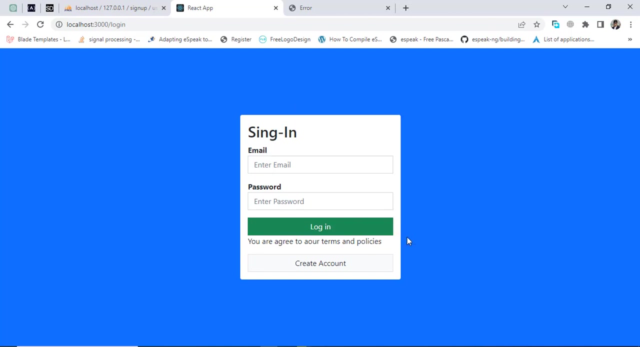 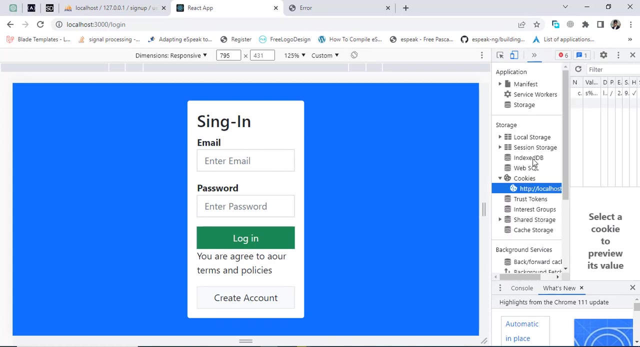 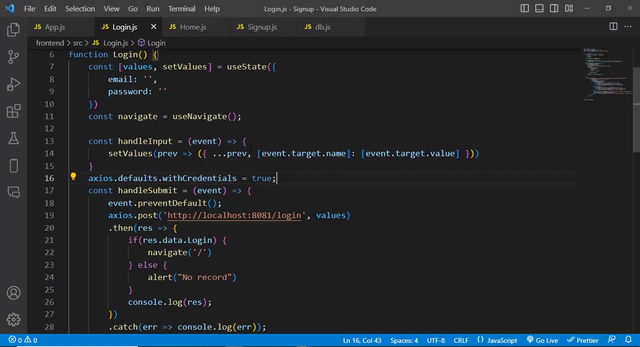 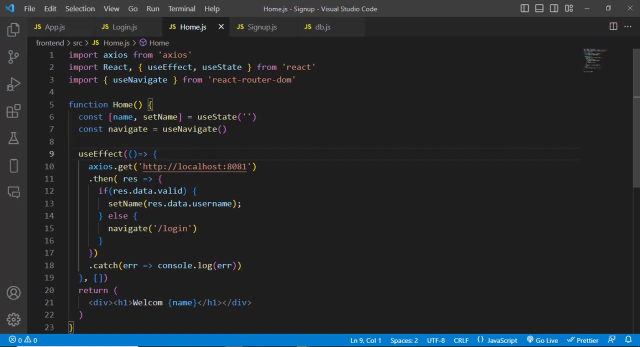 it. yeah, so whenever we log into our system for its login, see the message has printed for us. so let's appreciate again. session has gone. the cookie solids come here that we have the cookies are not. yeah, we have the cookies, we have the cookie. so let's check it. and here is the pie result: at it at a toilet. 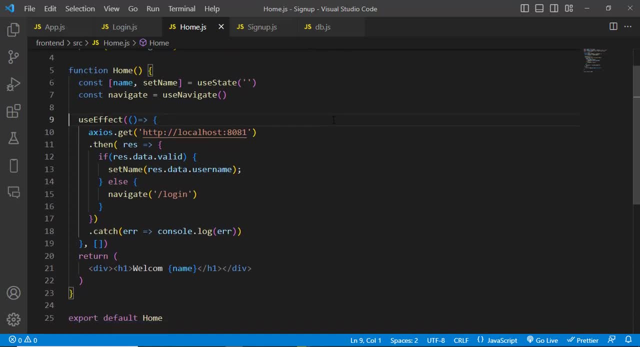 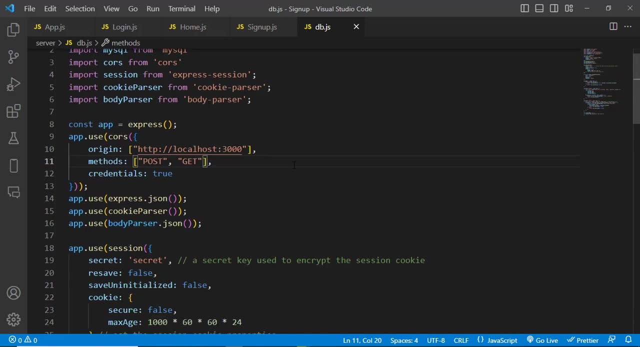 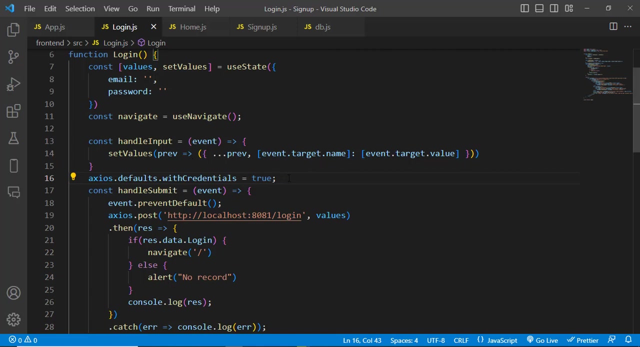 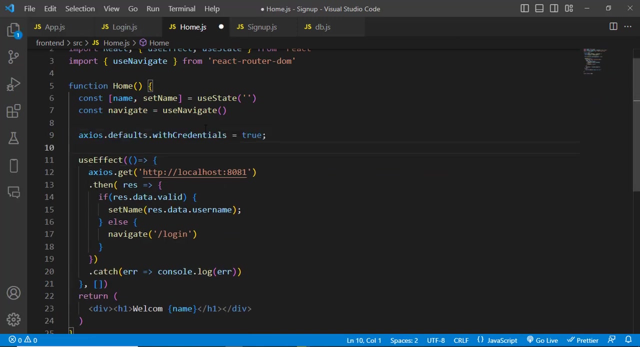 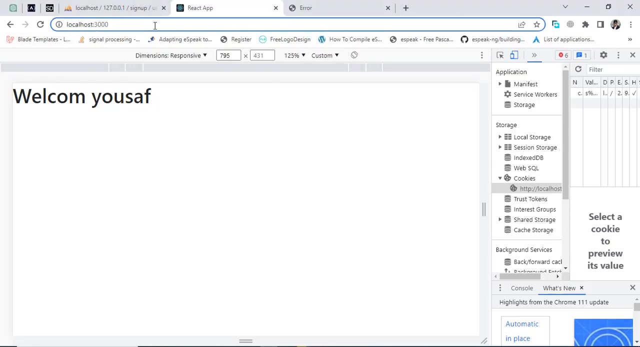 everything is okay. let's check it. login. so let's copy this access to default that credentials. we should specify that in home page also, because we are accessing with this route also. okay, so let's check it now. let's back to the login. let's appreciate again. 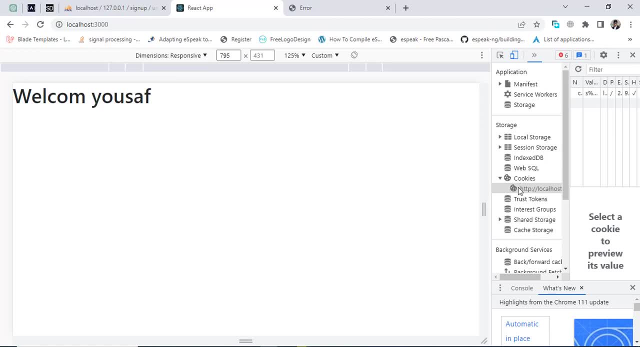 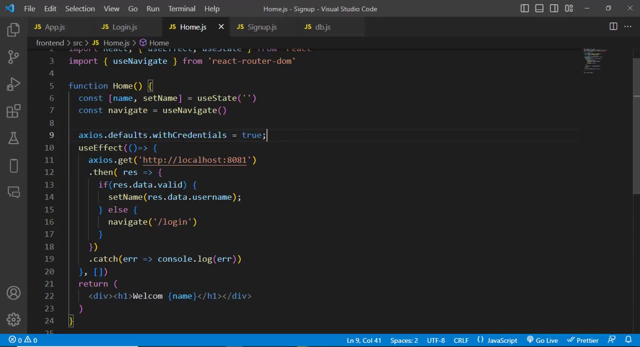 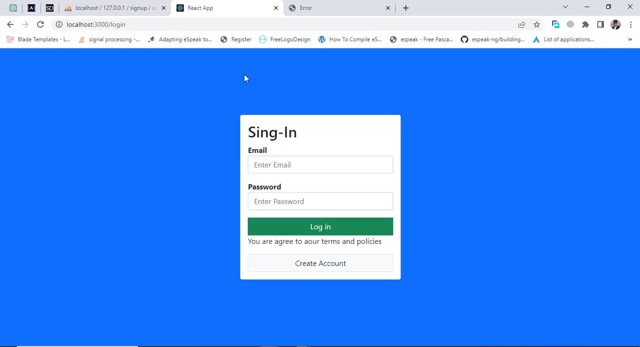 yeah, it's okay. it is printing our values for us in that. so we have the cookies, it all the cookies are okay, but before we were not, we didn't use this axis. the deport with the credentials. okay, if you would like to go to login now. so every still should specify if. 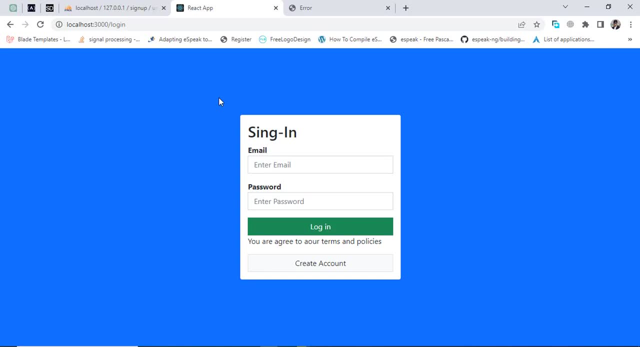 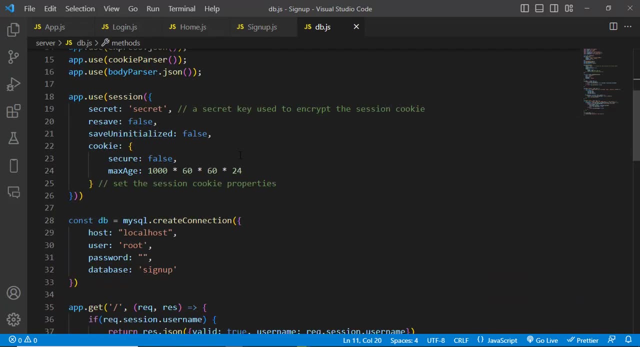 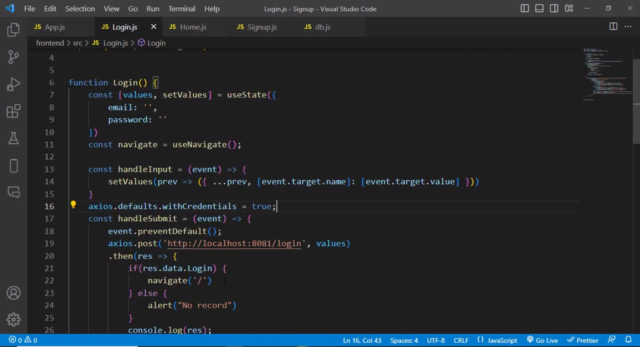 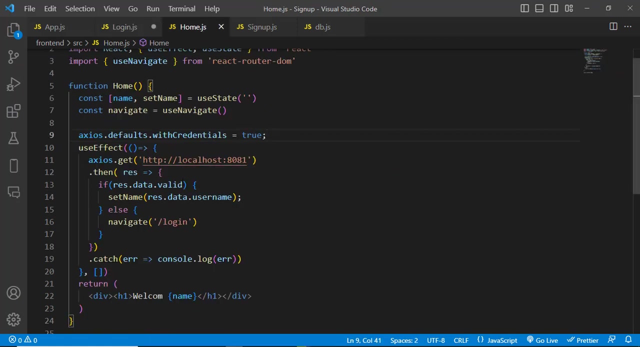 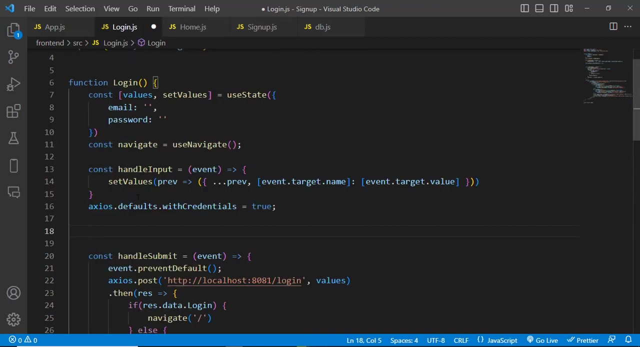 you were locked in, it means that the cookies were seat. so we should go back to our home page. Let's perform this in the like in section. here we should specify use effect also. Let's just copy this use effect. copy this, paste it here. we should move to home page and in result, a data wallet. if you were wallet. 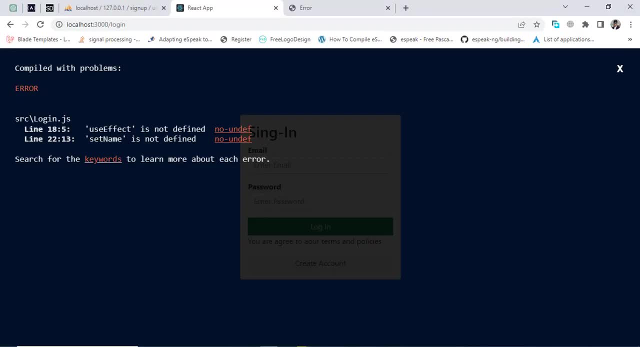 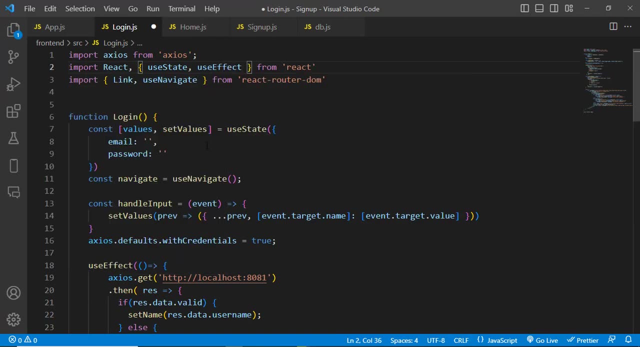 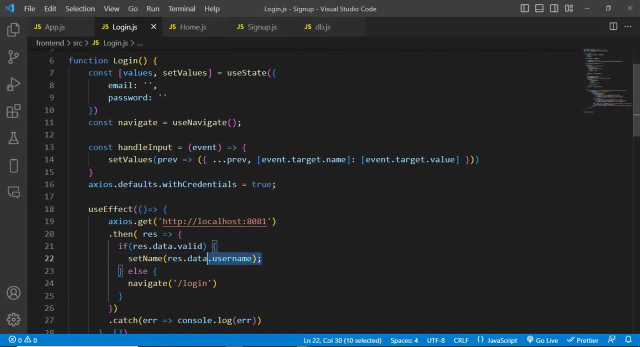 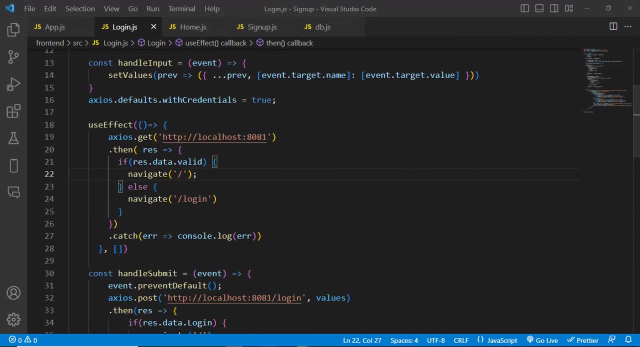 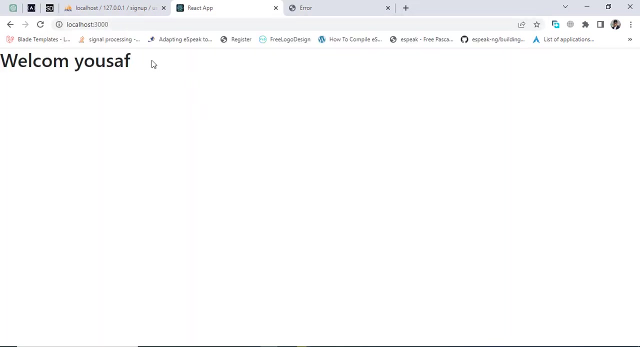 so it will be okay. if not valid, then it should goes to: and let's import use effect. and also, another error was: yes, let's remove this shit name. If you were valid, so we should. goes to navigate page. yes, let's check it now. So let's try to login because we are already logged in, so we